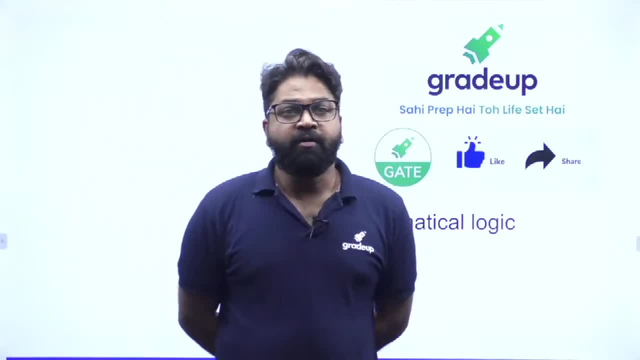 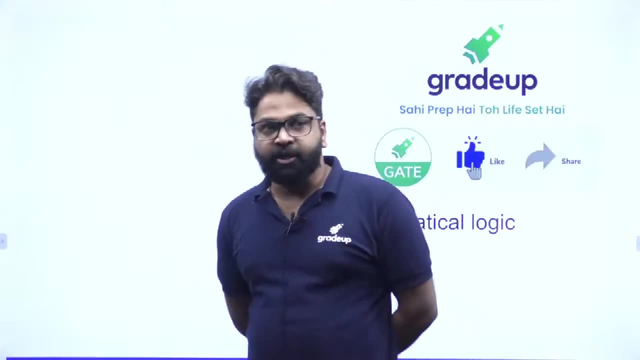 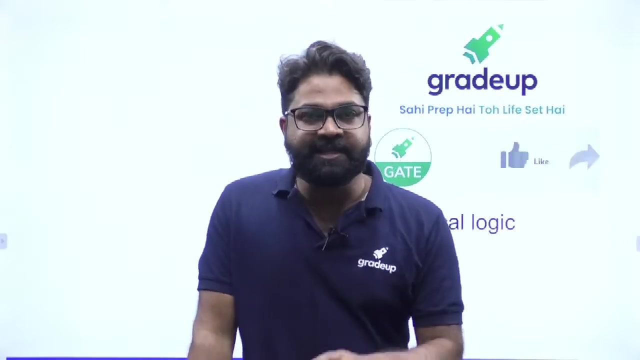 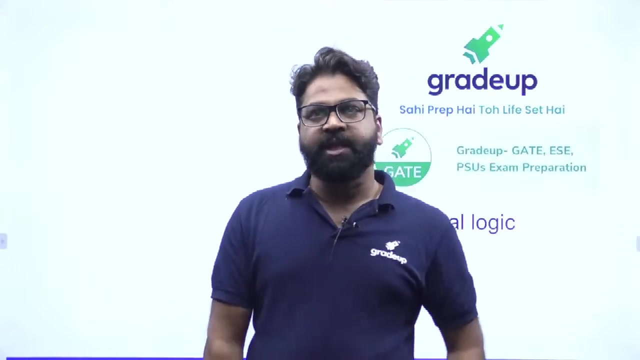 in, in, we can say that- into normal life, or what is the exact? you can say that you know the application of a mathematical logic. So today we'll go and we'll talk about that particular concepts. that is related to mathematical logic. So here I welcome to all of you on this, India's largest e-learning platform, grade up. So we'll go and we'll talk about the today's topic. that is nothing but mathematical logic. But before that, let me tell you about myself. My name is Satish Yadav. People also. 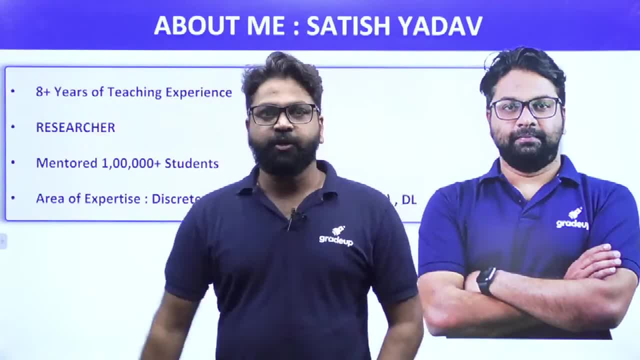 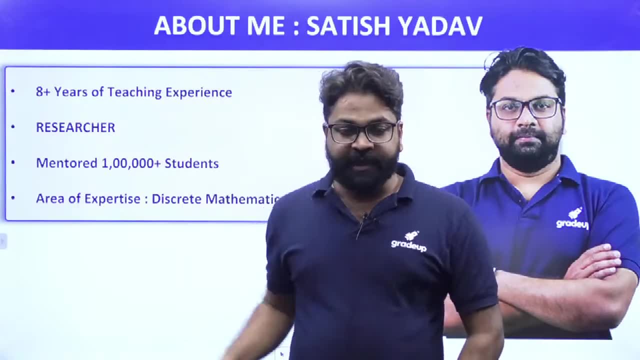 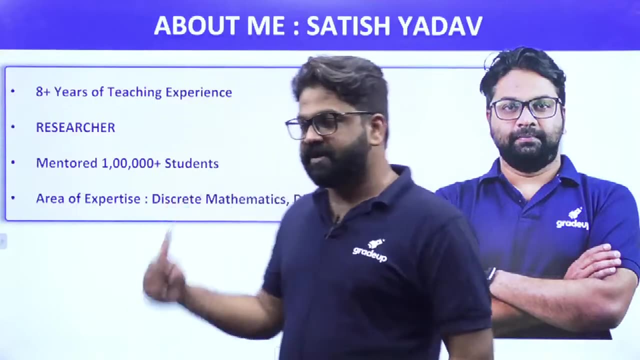 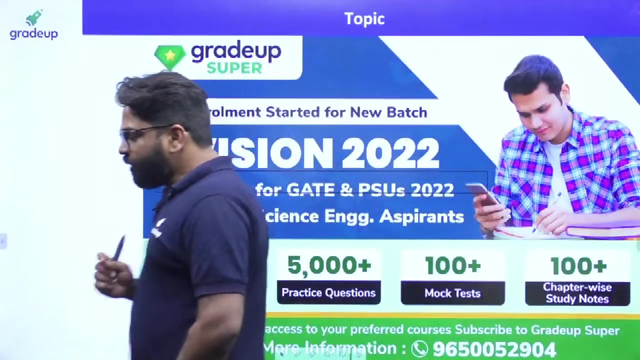 called me researcher or Baba, because I have done a lot of research into a different areas of a computer science and I have taught more than one lakh of students and throughout the whole India- you know across all the cities- and my areas of expertise are discrete mathematics and you can say that DBMS. So we'll go and we'll talk about the mathematical logic, But before that let me tell you about the grade up, super subscription. See many times the student. 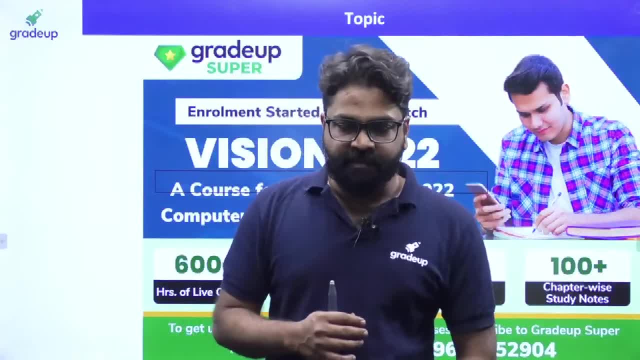 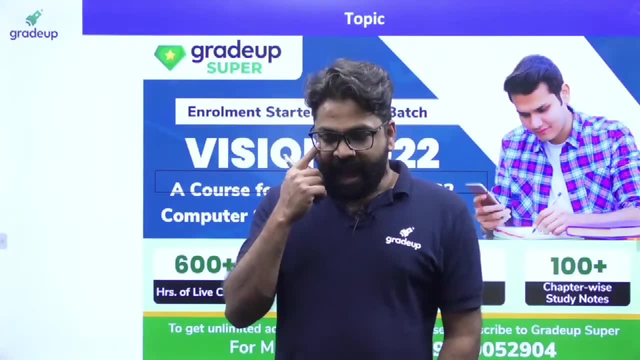 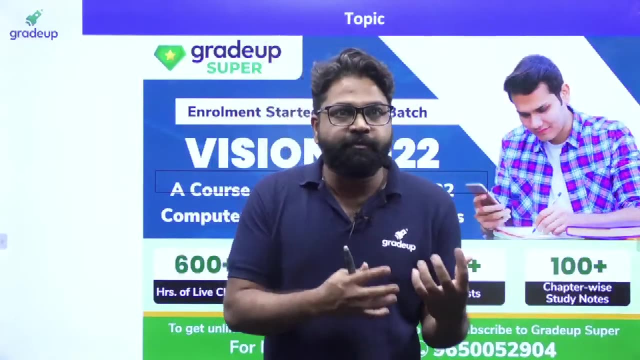 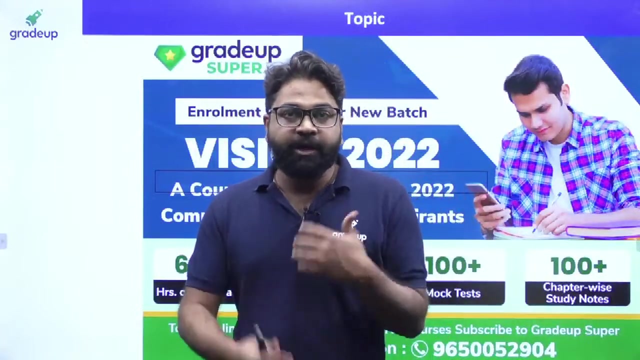 are they want to prepare for a particular examination. Suppose, if you want to prepare for a particular examination, then what will happen? you think that I will prepare for this particular examination, but I am not getting a proper structure schedule. I don't know from where what to study. I don't know which type of reference book I have to use, or what type of concepts that I have to grab, or what type of questions that I have to solve, or what are the quizzes that I have to take. So, in order to do that, 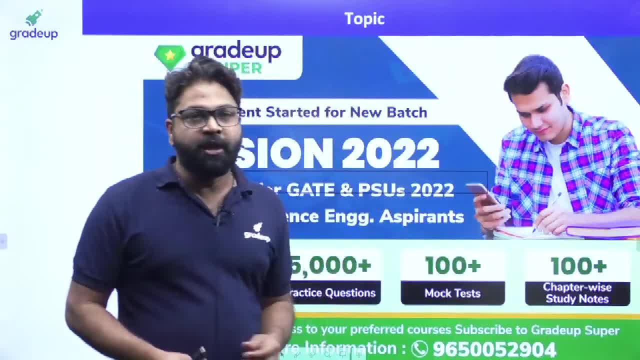 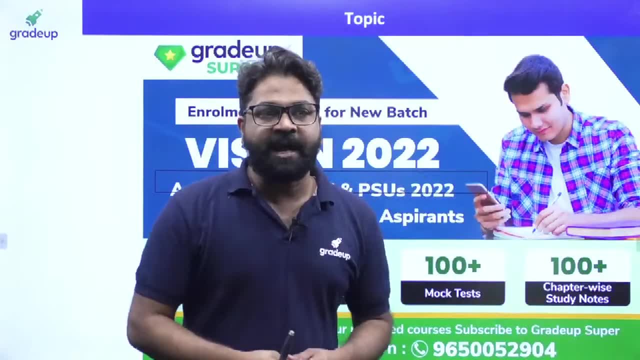 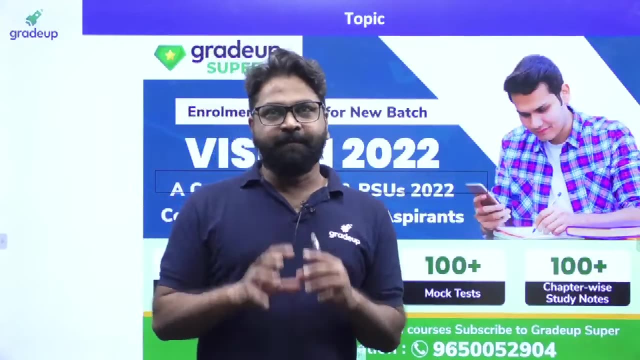 that here the grader is providing the super subscription so that your plan will be structures. so for the whole year the grader will giving you this particular plan, okay, so that you can watch this particular type of what the plan see. for example, if suppose, if someone says that i am 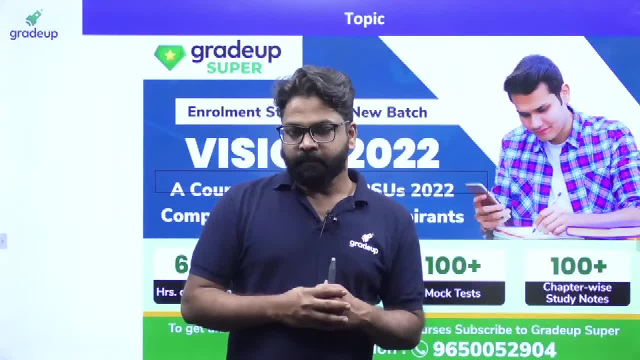 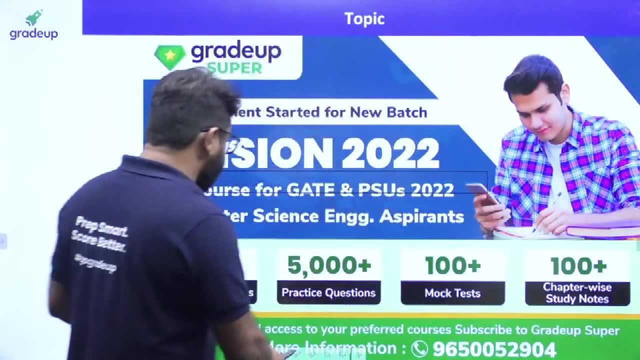 going you or i am providing you. let's consider a suppose: if i am providing you the whole year plan or the whole structured plan or something like that, then the grader is providing you that. so see, what are the advantage of having the grader subscription? you will be having a 600 hours of. 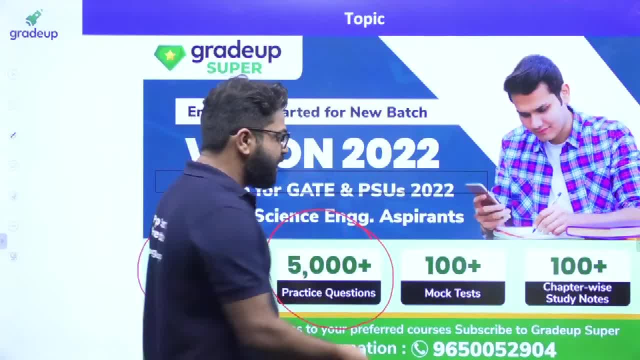 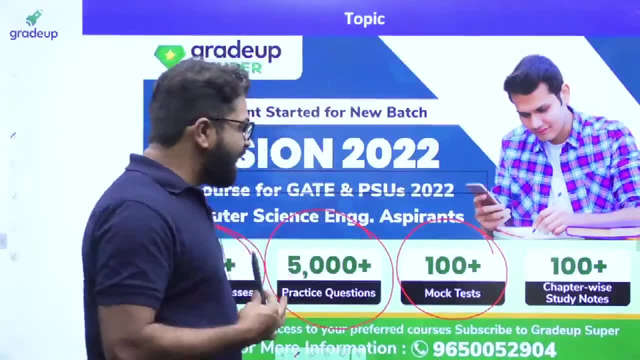 life classes. you will be having a 5000 of a practice questions. you will be having hundreds of mock test. you will be having the chapter wise notes also. you will have the quiz also. these all are the advantage. that is related to what. that is related to grader super batch subscription. 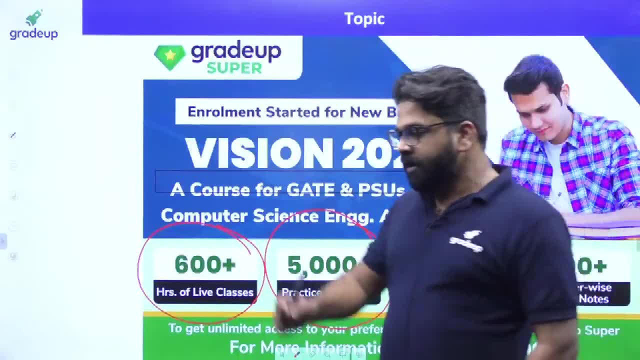 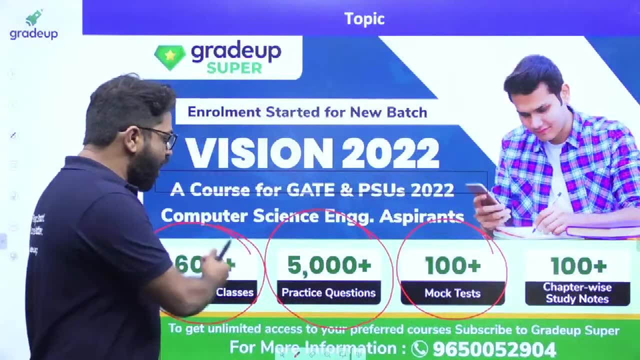 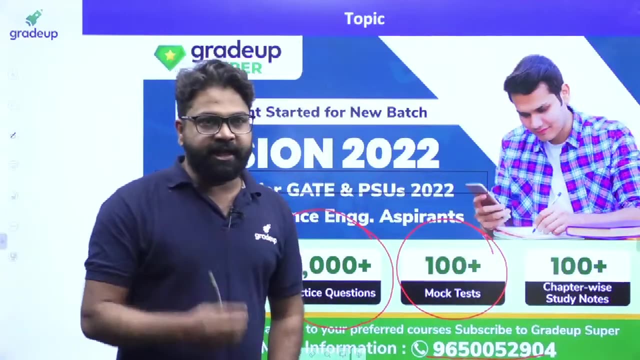 so once you will take a grade up super subscription, the advantage that you people are having is basically what the advantage that you people are having is basically you all are getting this extra things now in order to take the subscription. you can contact on this number and i'm sure our team will be assisting you in a best possible way. 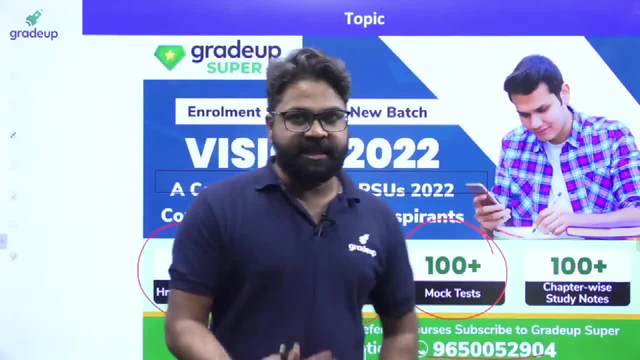 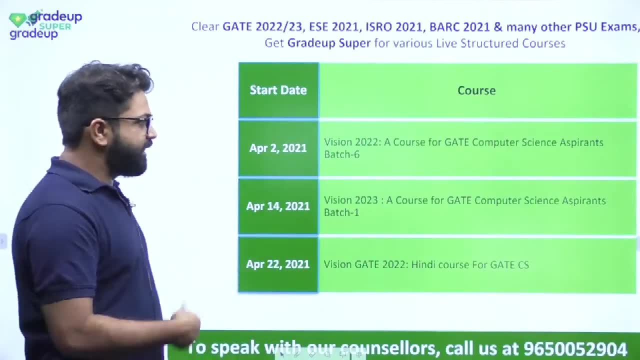 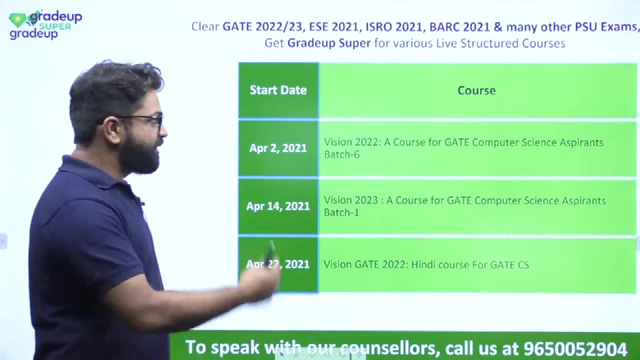 so 9650052904. that is nothing but the thing. anyhow, if you want to understand about the other batches, what the grade up is coming and what the grade of will be teaching, so here the upcoming batches will be there. okay, the already the batches are going on, but still you can enroll for the other. 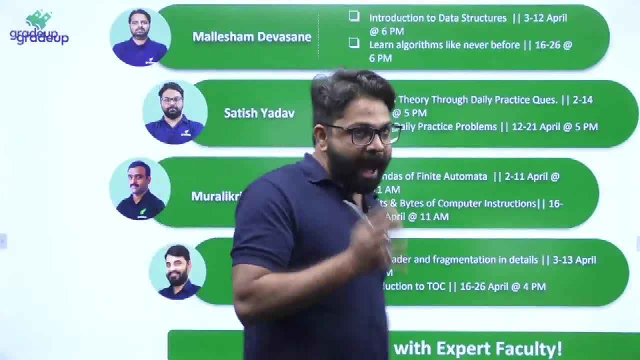 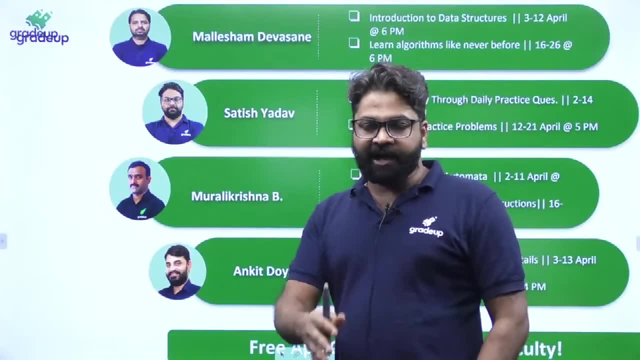 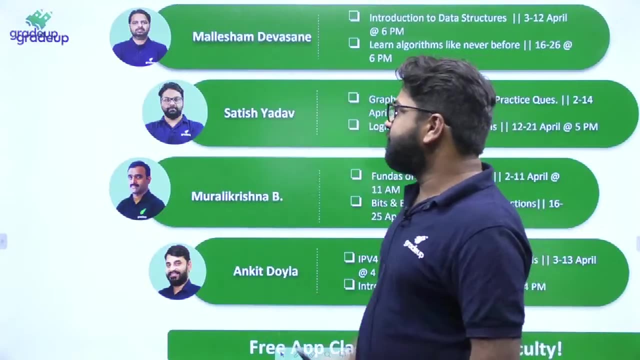 batches. now, if see on a grade up app also. so those people who have not downloaded the app, you can also download the grade up app, because in grade up app we are teaching most of the times the free sessions- okay, over here without subscription. so here the sir is taking which. 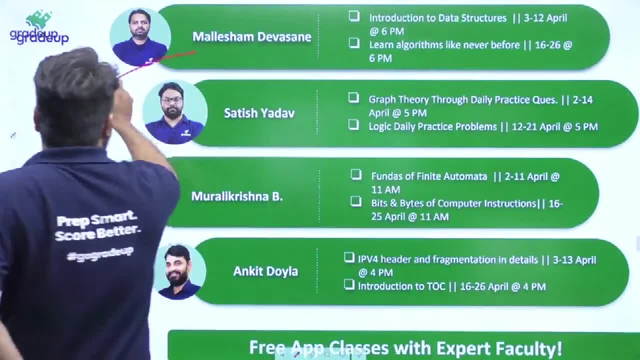 is nothing but everyday class. so you can see that here the sir is taking the class at 6 pm. i'm taking a class every day. you can see that here the sir is taking the class at 6 pm. so you can see that here the sir is taking the class at 6 pm. 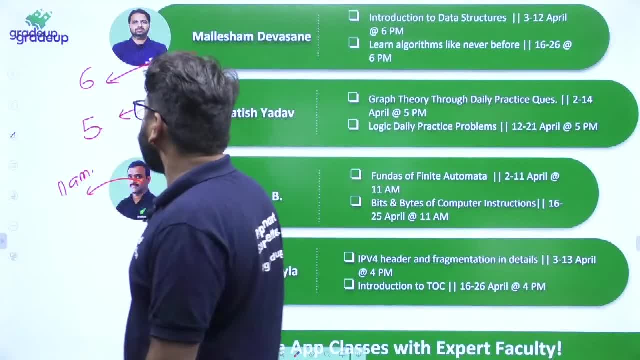 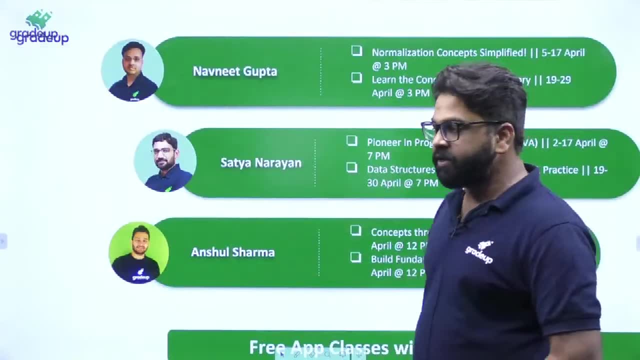 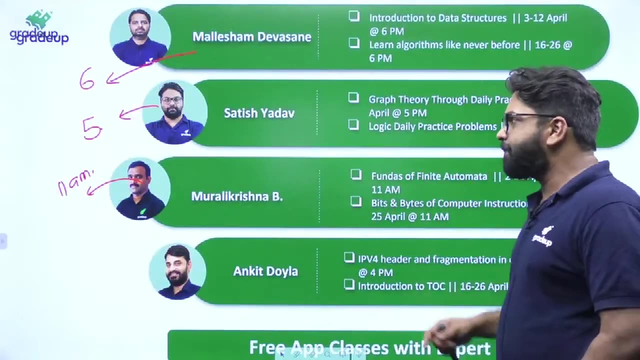 the sir is taking the class at 11 am. okay, so all the faculties, all the you know the experts faculties are taking the classes. you can note down the timings also. okay, suppose, if you want to do a practice with respect to my subject, so every day 5 pm on a grade up app, you can come. 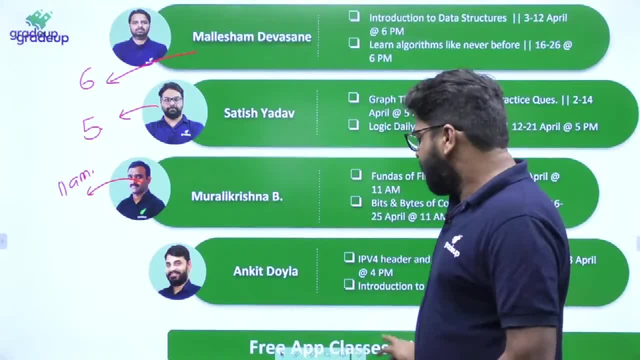 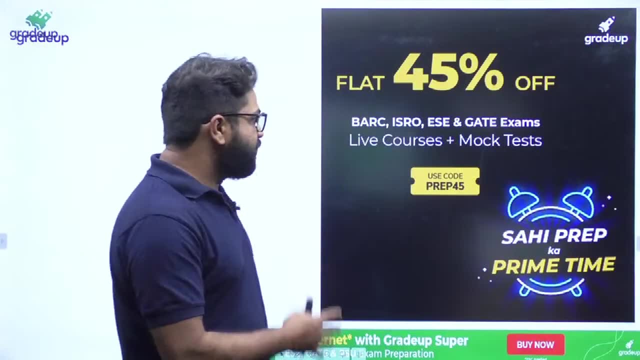 and you can join me. yes, today also, you can come and you can join me. okay, this all are the advantage and here you will be having one of the benefits that you people are getting with respect to you. if his time, your roaming time, however, what happens is you will find student are. 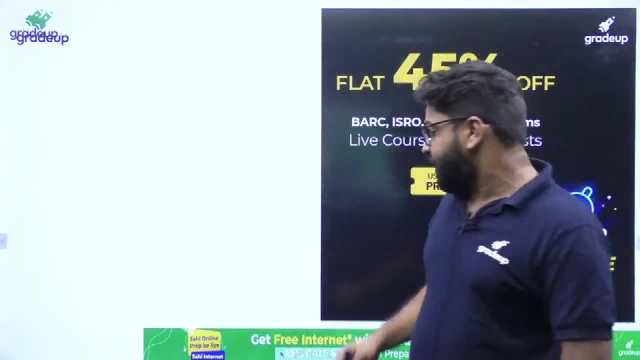 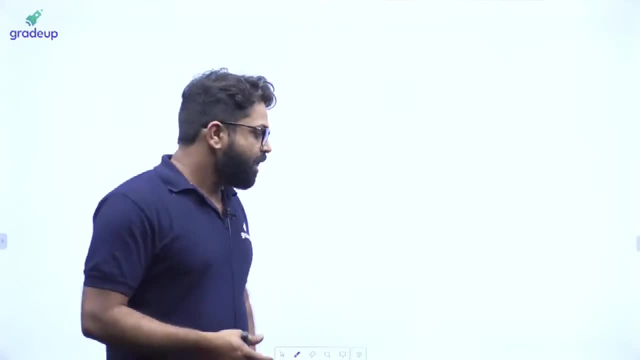 not covering us because student are 对 in. you know, Watson is taking fkay V Bugün. he is okay, the people listen to me, we always36.. any, how will go and will start. okay, we'll go and will start. which is nothing, but which is nothing. 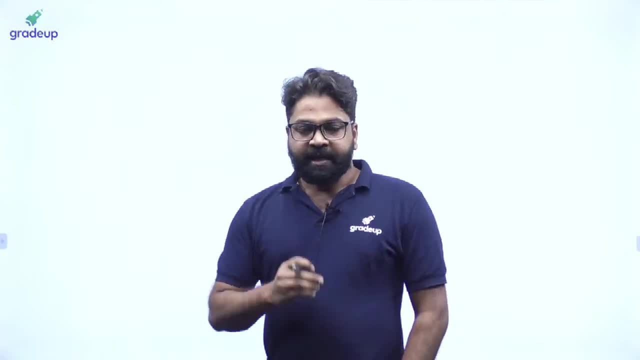 but that I get a no. okay. so here we will go and we will try to start, which is nothing but mathematical logic, and we'll talk about what is a mathematical logic or what is the application that is related to that. see, many times the student used to ask me: what is the mathematical logic? 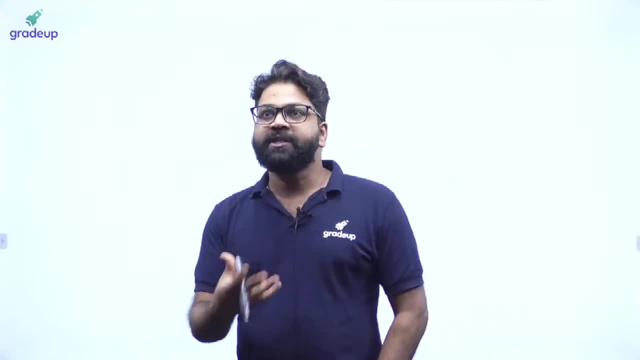 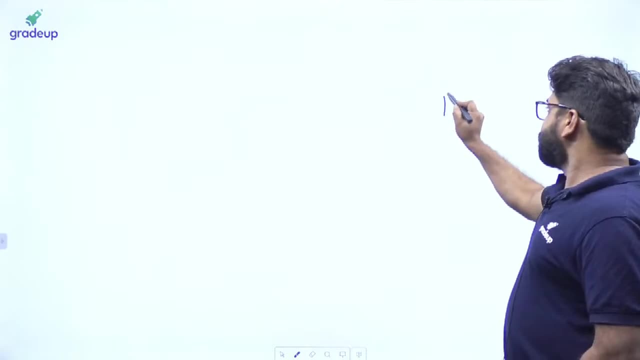 logic or what is. you can say that the concepts of a mathematical logic or why it is used into that. see. most of the times the students are saying that see, you are having which is nothing but programming language and from a programming language, what you will do is basically, you are. 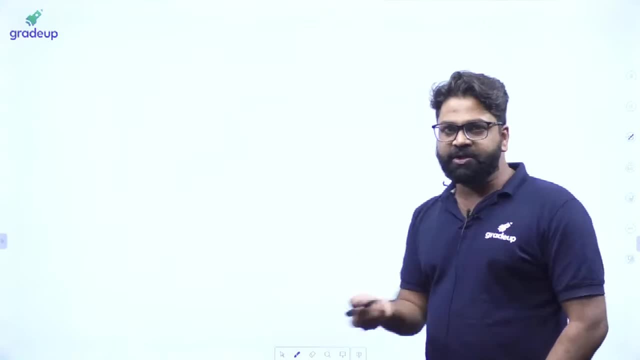 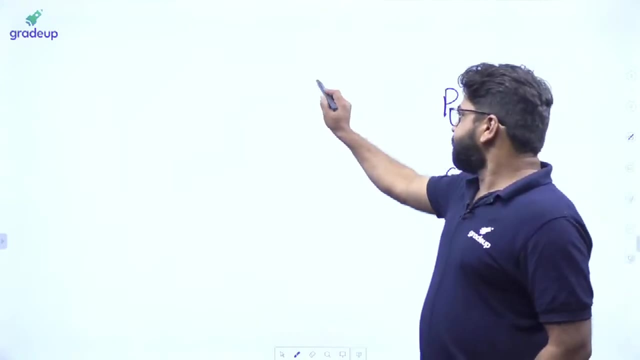 drawing the software. so from a programming language you are making to a software, and then we are thinking the computer science is over, but the computer science is not over. there are various things into that. first of all you should be having the algo, and then from algo you will be. 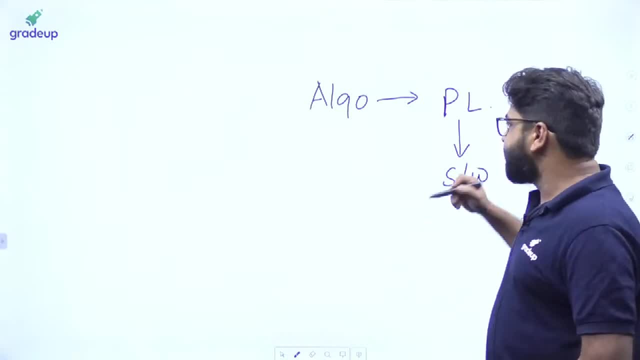 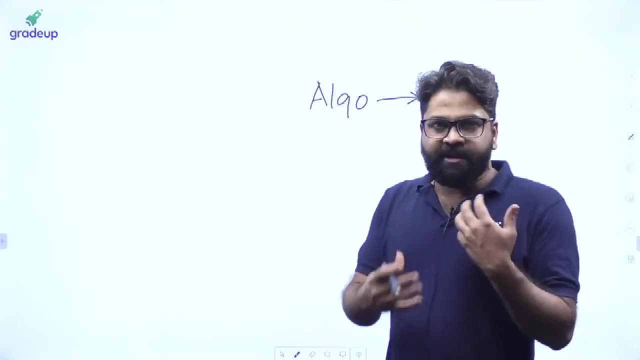 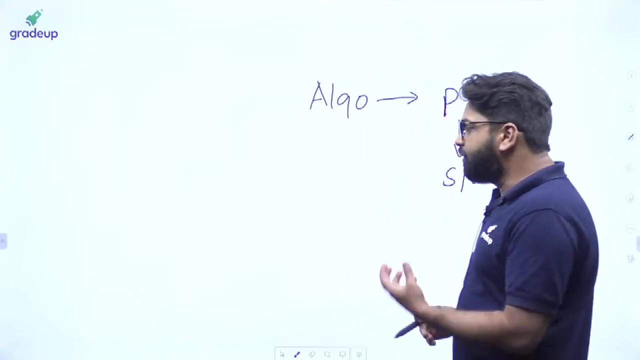 having the programming language and from programming language you will be converting to software. but obviously we cannot use the algorithm as it is. see, suppose if I, if anybody is saying that, can you draw this particular software. so what you are doing is basically: first you should know the algo. 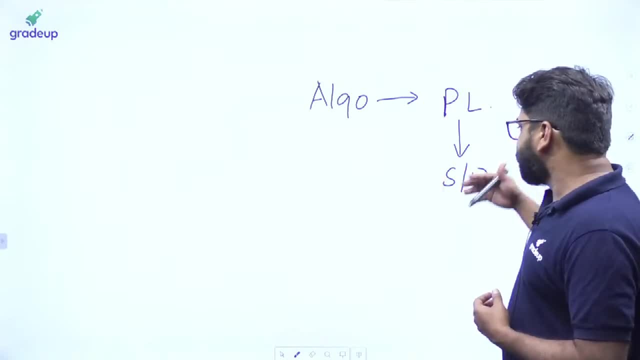 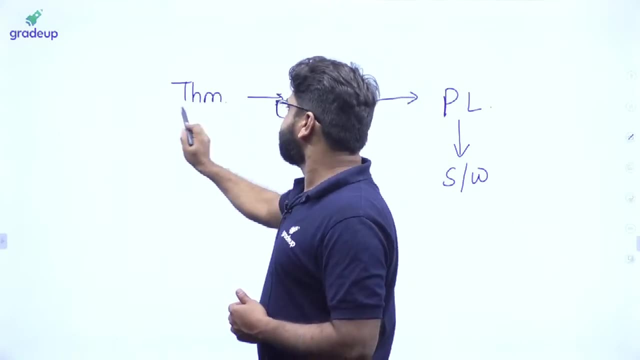 and then from algo you are using into programming and then from programming you are making into software. but in order to use the algo you are making into software and then from algo you are, you should have a theorem. okay, you should have a theorem, but, sir, where is? 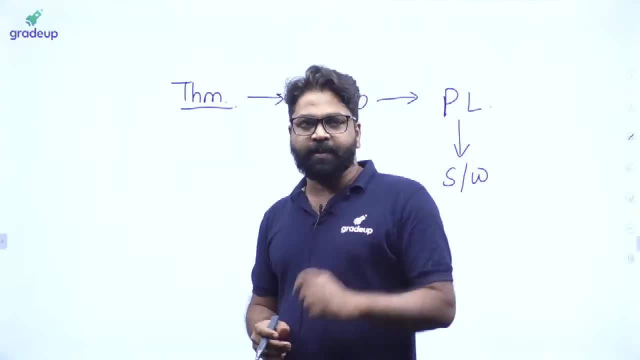 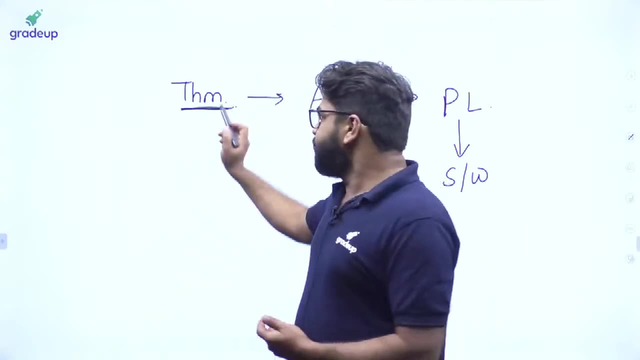 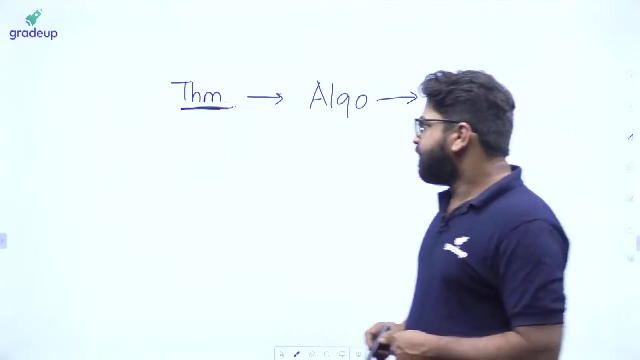 this mathematical logic, the mathematical logic that you people are having over here, is basically in order to prove the theorems. so once you will prove the theorems then you can use into the algo and then you can use into PL and then from PL so you can have a software. but theorem is not just a state forward. 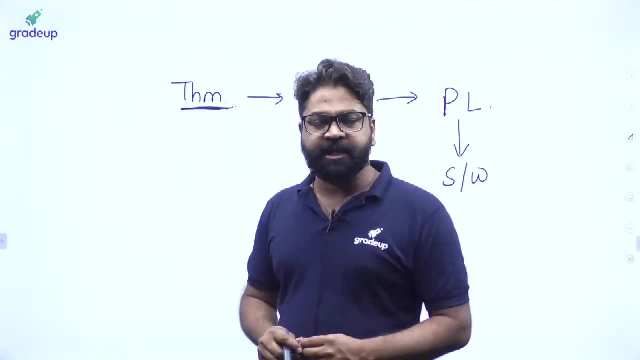 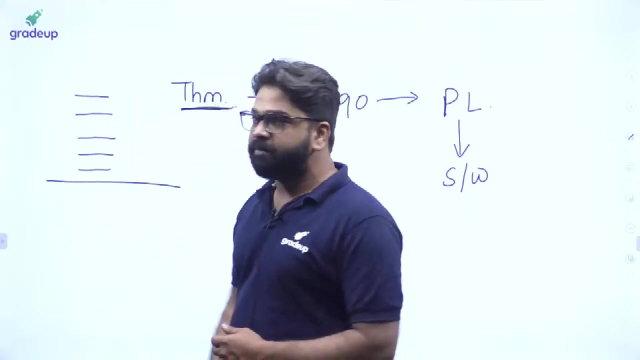 statement. theorem is not just a state forward statement in order to prove the theorems. there are multiple statements that leads to a single statement. there are multiple statements- see when we are deriving- or any particular theorem. so there are multiple statements that leads to one statement and that is called as. 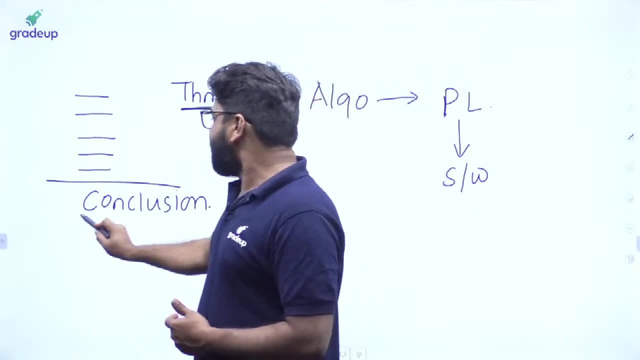 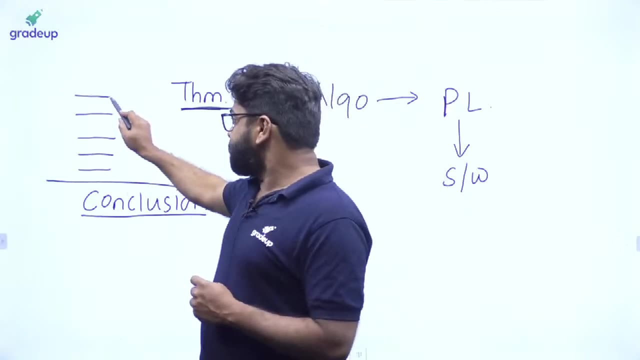 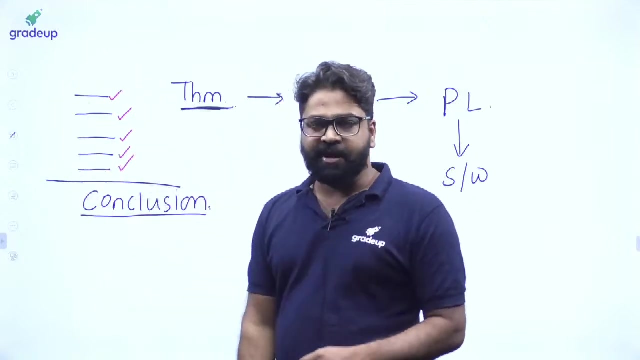 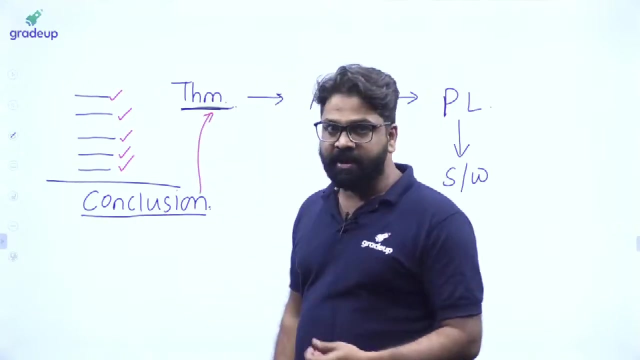 what that is called as a conclusion. so here what you will be having, here you will be having the conclusion: okay, now what will happen. see now what will happen. This is one particular statement. This is another particular statement. another particular statement, another particular statement, These all statements leads to a one point that is called as what that is called as a conclusion. Now, this conclusion is called as a theorem. Now, from a theorem, theorem to algo, algo to PL, PL to software. 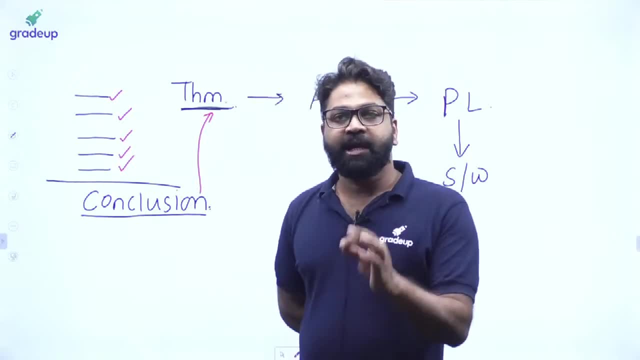 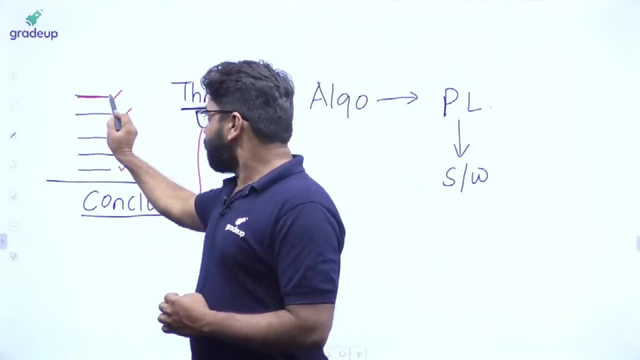 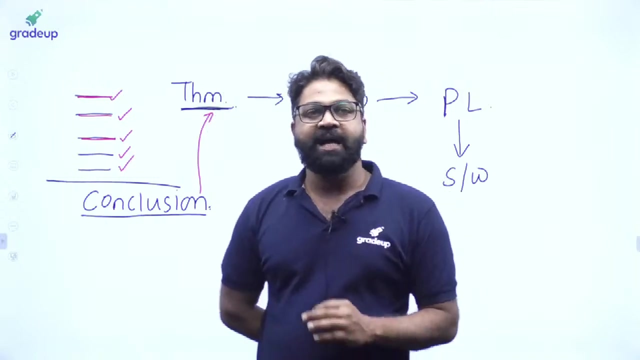 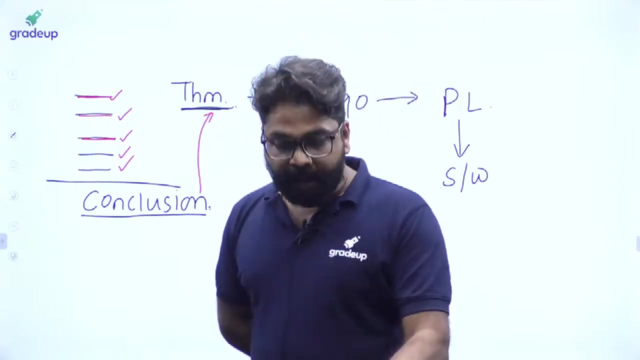 Sir, where is mathematical logic? Mathematical logic, it gives us power. mathematical logic, it gives us power to check the validity of this statement, to check the validity of this statement, to check the validity of this statement. So, if anybody will be asking what is a mathematical logic or what is the real time application of mathematical logic, then you have to say that a mathematical logic, it gives us power to check the validity of this statement. 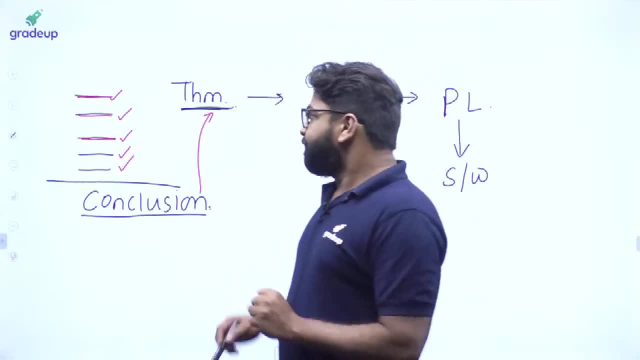 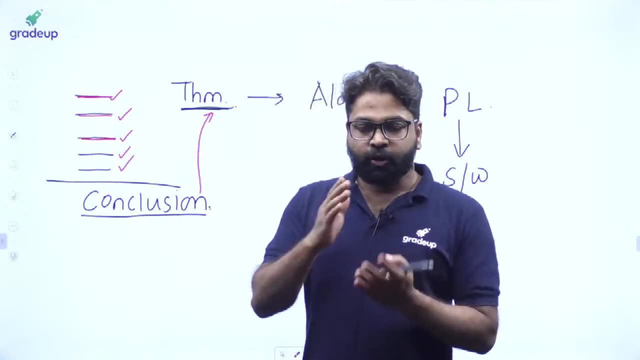 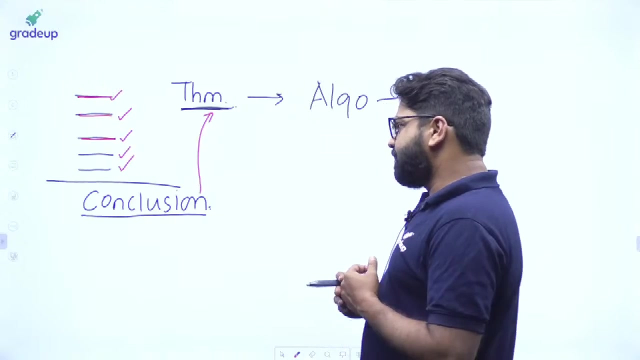 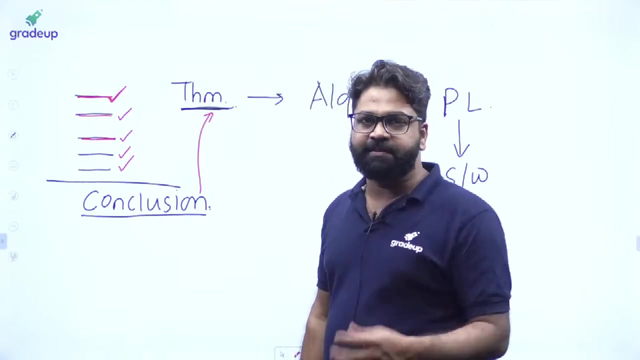 So to check the validity of a statement. So most of the times when you will learn about a mathematical logic, it gives you power to check whether this theorem is valid or not, to check whether this statement is valid or not. Now I, okay, sir, I got the. you know the why we are learning the mathematical logic: to check the validity of a statement, whether to check the statement is valid or not. Okay, So that is nothing but the main concept why we are learning the mathematical logic. 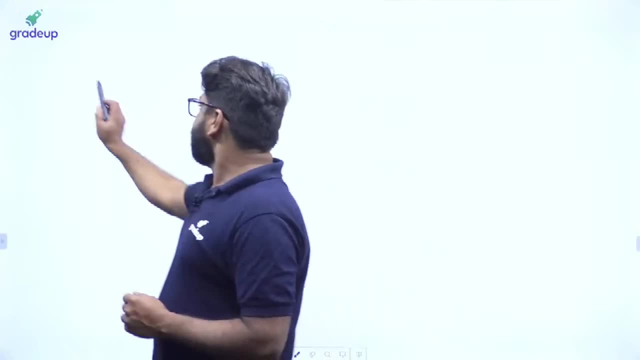 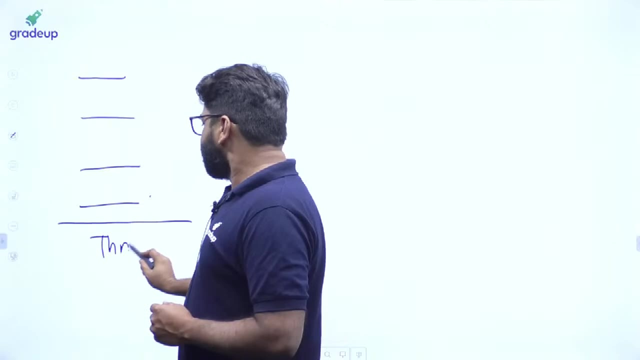 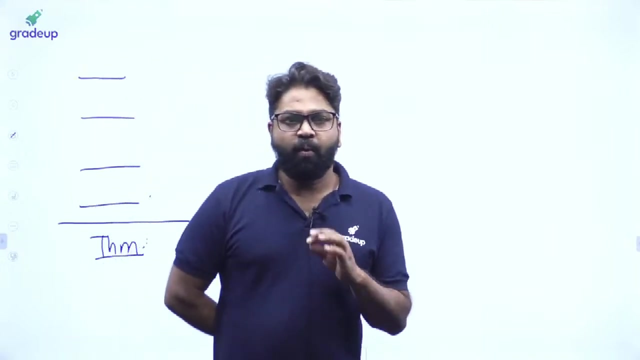 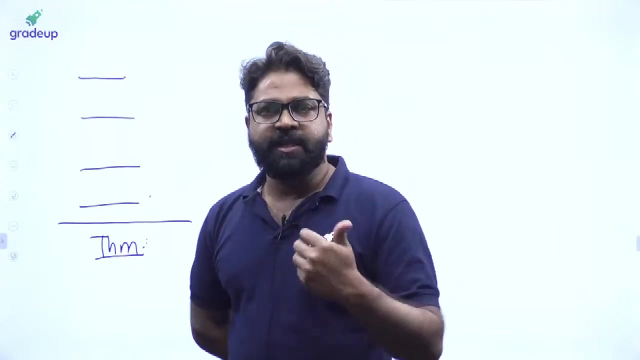 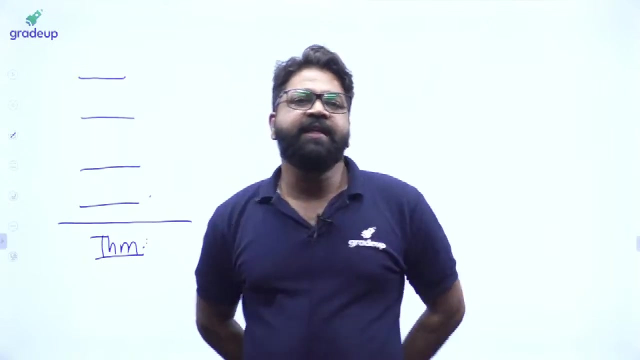 Now here we'll go and we'll talk about this particular Statement. See if I will be having which is nothing but this type of statements here And here you will be having a theorem. So I'm not getting how you are writing the statements and then you are writing the theorem, Okay. Now what I will be having is basically, if I will say that, okay, if I will say that, suppose in in 10th grade or in 8th grade or something like that, then what you are writing is basically, you suppose, if somebody says that, prove that sine squared. 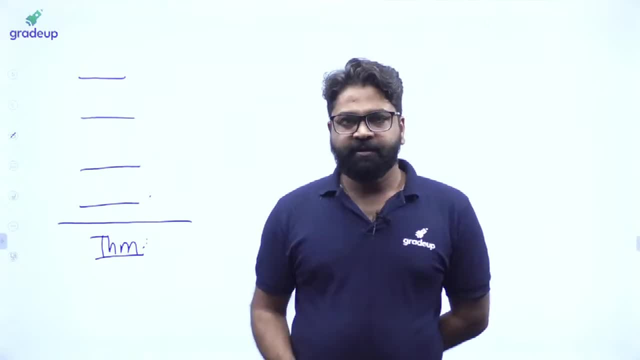 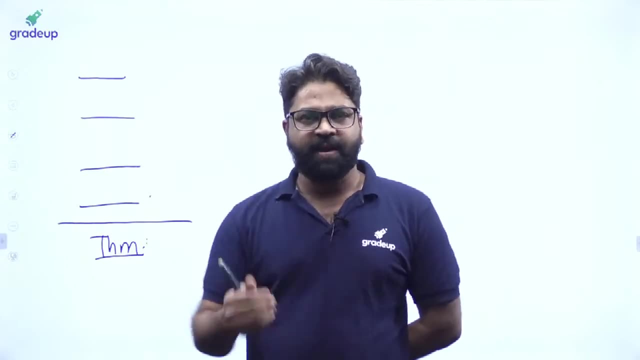 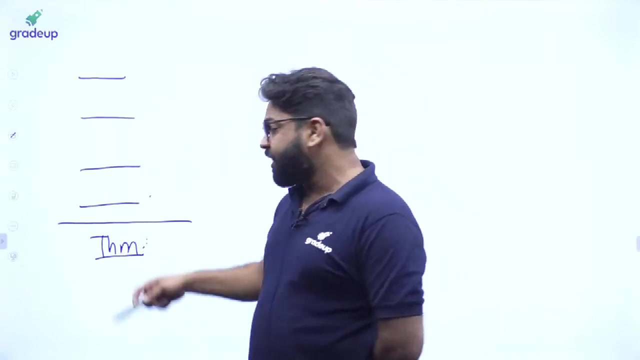 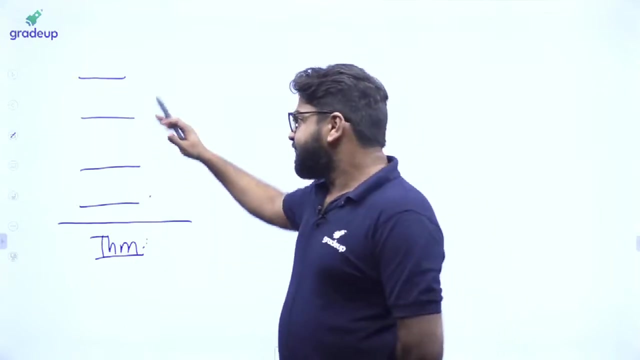 X plus cos square equals to one, Then you cannot directly prove that. So, yes, what you are doing, you're writing the steps. You're writing sine 30 something. You're writing cos 30 something, And then you're writing sine square 30 equals to something. You're writing cos square 30 goes to something And then you are proving- My point is theorem in order to prove the theorems. We are not directly proving the theorems, but we are writing, you know, multiple statements and then we are proving it from where we are taking the statements. We are taking the statements not just randomly, We are taking the statements. 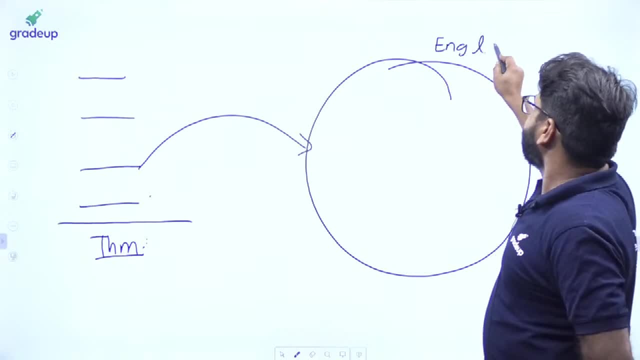 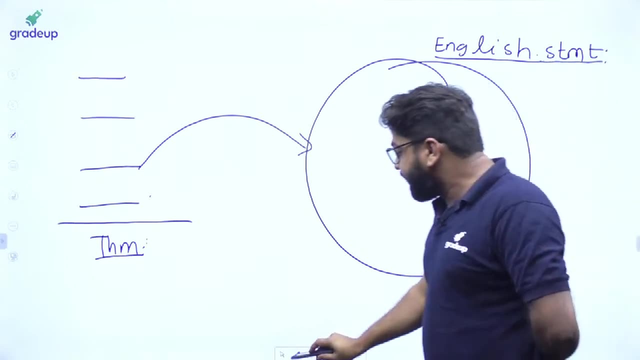 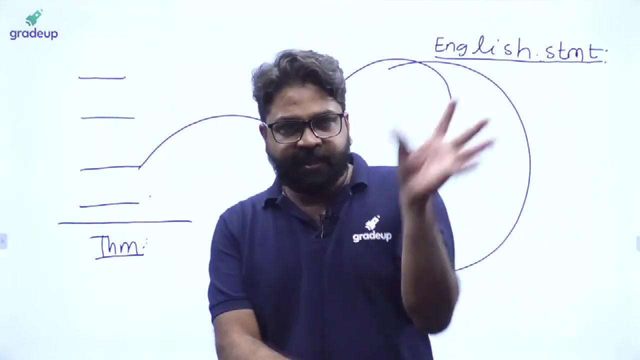 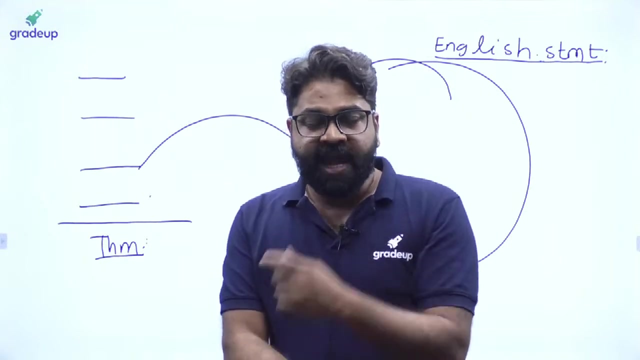 We are taking the statements from a set of English statement. So here you will have what? here you will have a set of English statement. So here you will be having what? here you'll be having a set of English statement, But again in a set of English statements we there are certain different types of statements. If there is a set of English statement, there is a different type of statements. There is a ordering statements, There is a, you know, questioning statements, exclamatory statements, imperative statements, But we don't take all the types of statements. 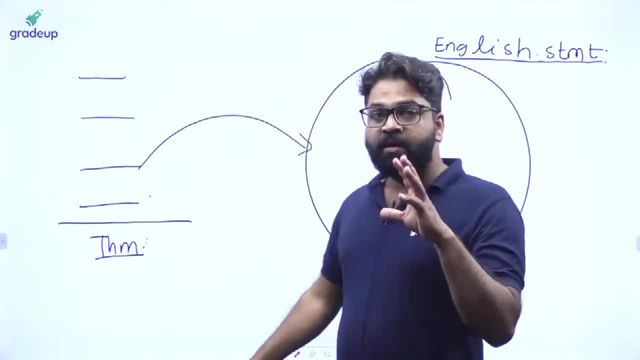 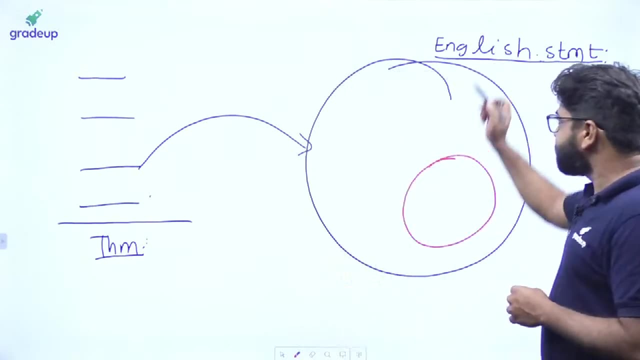 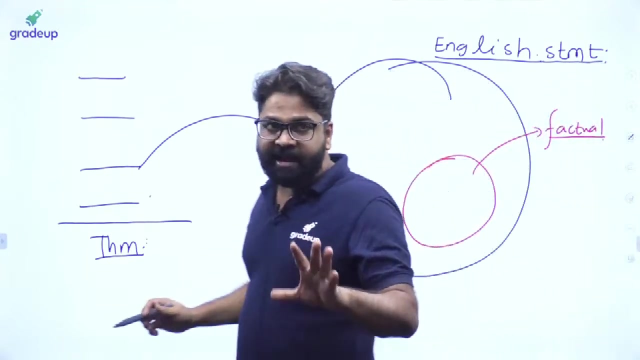 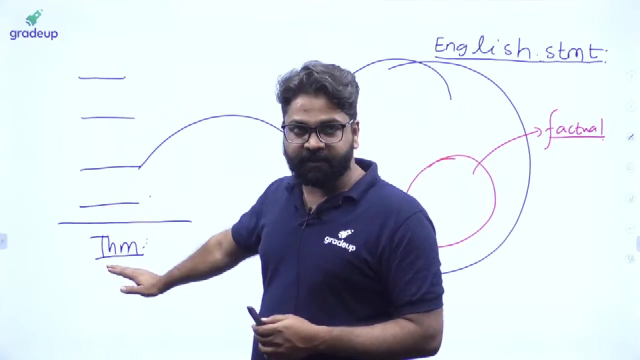 We are taking the statements into in order to prove the theorems. We are taking a selected type of a. you can say that selected type of a statements and that statements. that comes from English statements. Those type of statements are called as a factual statement. So we are not see again. I will go in again. I will tell you We are having the statements based on the statements. We are giving the theorems. These statements we are not just taking randomly from here. We are taking the statements. 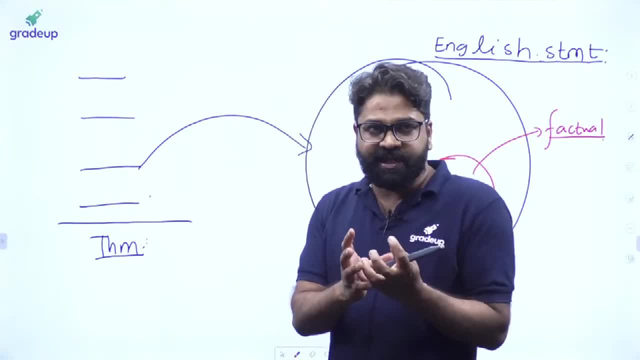 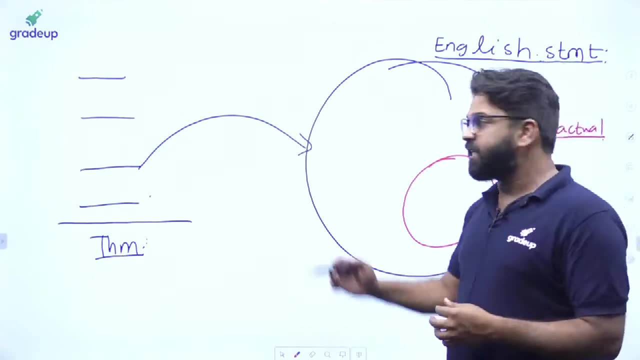 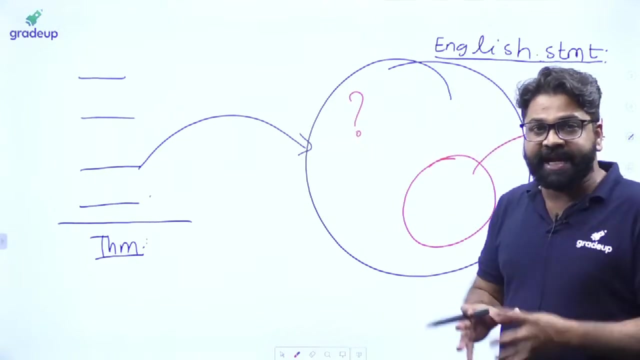 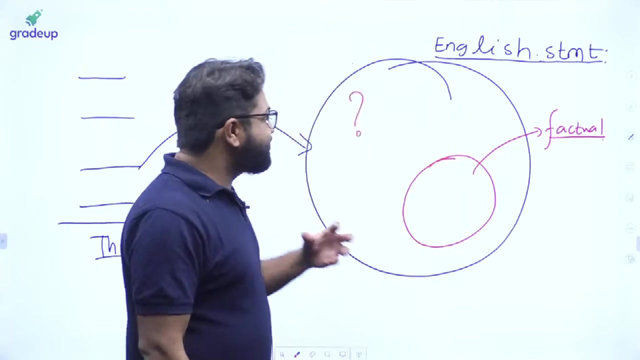 We are taking the statements from a particular set and that set is called as what that set is called as a factual statements. This set the English statement. It is made up of different statements. It is made up of questioning statements. It is made up of ordering statements. It is made up of exclamatory statements. We does not take all the statements, but we take a selected, a type of what we take, the selected type of statements, and that selected type of statements are called as a factual statement. Now, if anybody asks what is a factual statement? 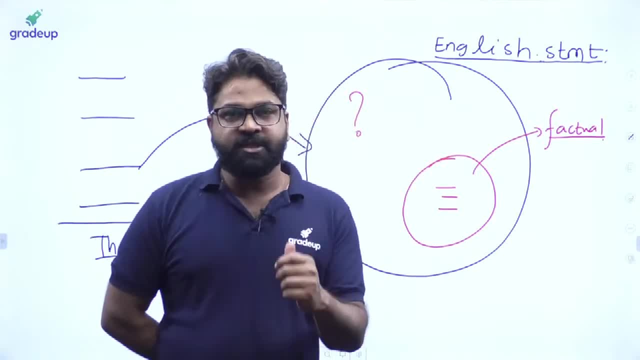 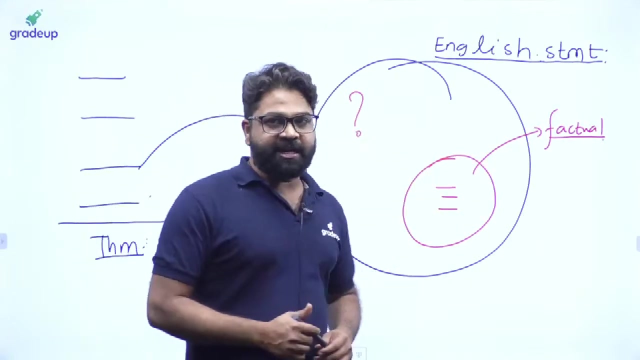 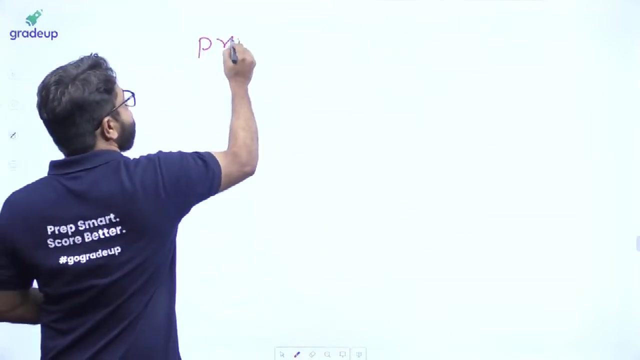 Then you have to say that a factual statement is basically a type of statements that defines the facts. What is that fact? The fact is basically either true or false. So here we'll go and we'll talk about. in mathematical logic This type of factual statements are called as a propositional statement. So here I am, having that propositional statement. So now we'll go and we'll talk about this type of statements and that is called as what, that is called as a propositional statement. 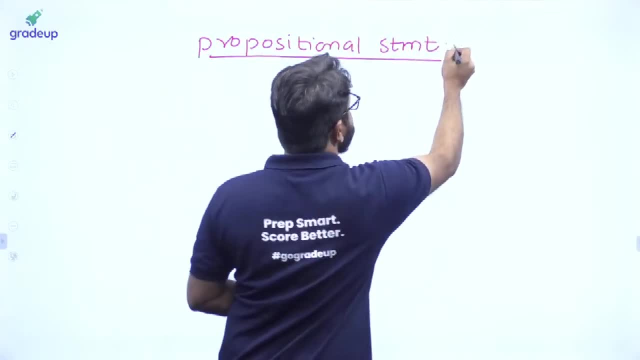 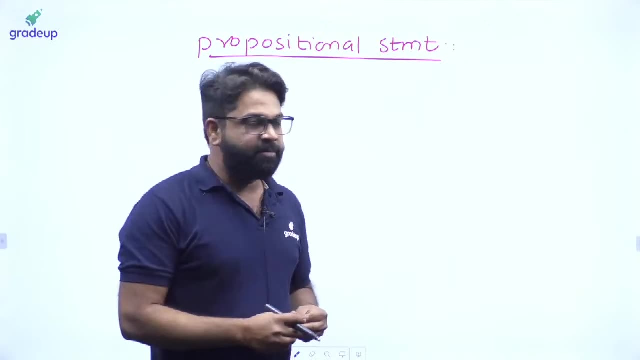 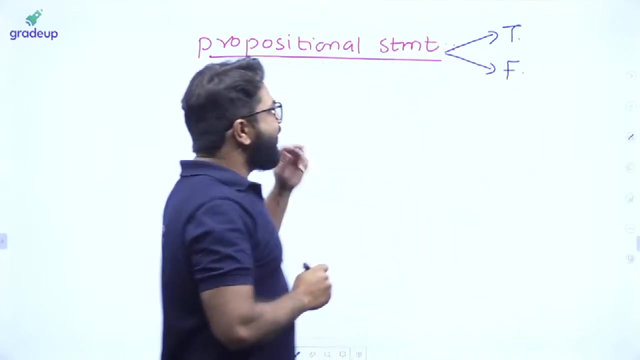 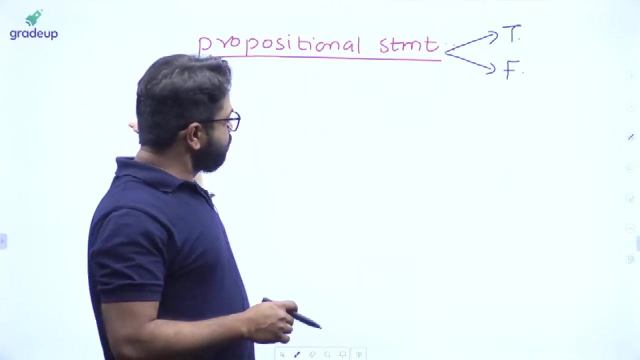 A propositional statement. It is a type of statements that defines the facts. As I told you, a propositional statement is basically- you can say that- a factual statement. So that defines some facts. Either it can be going to be true or it is going to be what it is going to be false. So either it is going to be true or it is going to be false. It defines some facts. Now, okay, sir, I understood your flow. but propositional statement, It is of two different types. One is of two different types. 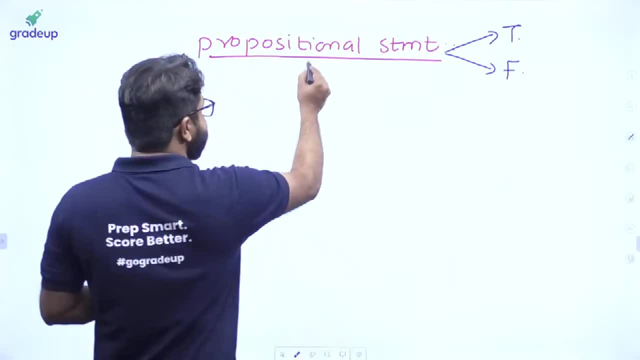 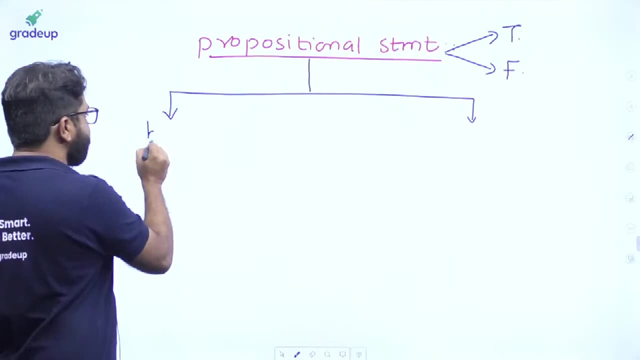 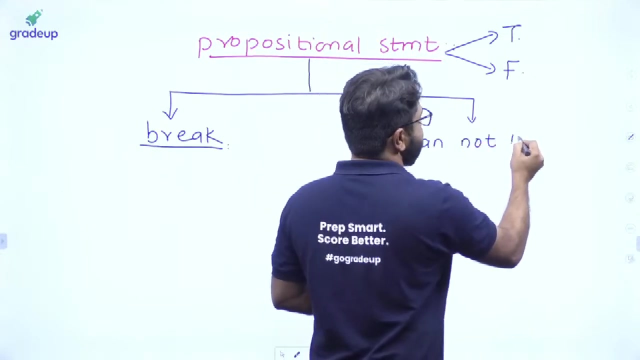 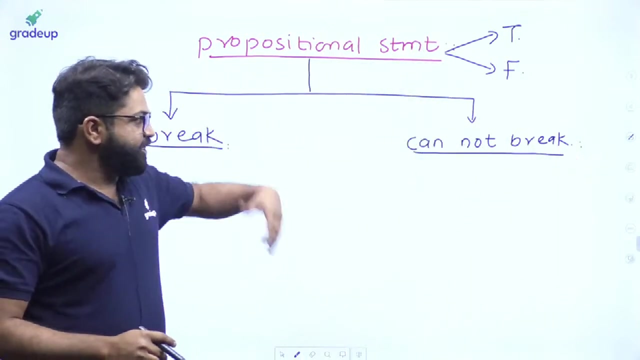 One you can break it, Other one: you cannot break it. So if I am talking about the propositional statements, there are two different types of propositional statement. One you can break it, One is breakable, Another one you cannot break it. Another one you cannot break it. Okay, another one you cannot break it. So one is called as what? one is breakable. Another one is not breakable. When it is not a breakable, that means you cannot. you, you cannot break it. That is called as a simple propositional statement. 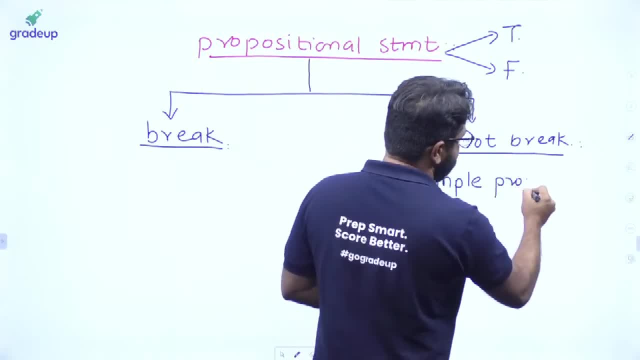 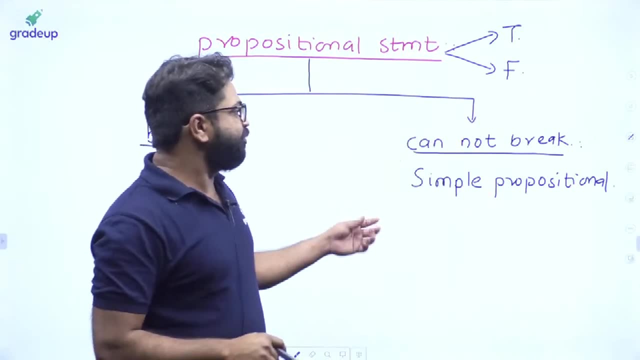 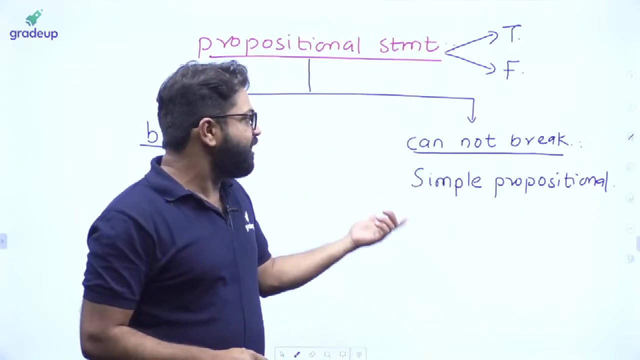 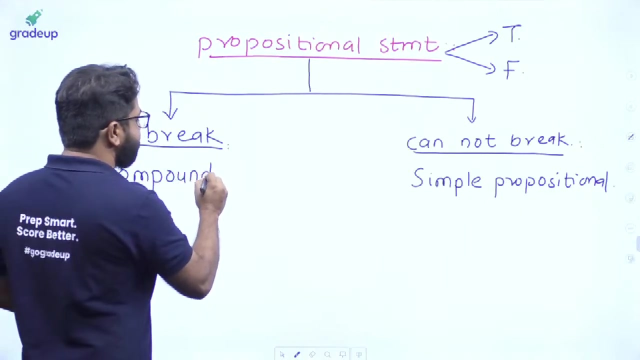 That is called as a simple propositional statement. Okay, that is called as what that is called as: a simple propositional statement. So if anybody is saying that what is a simple propositional statement, then you have to say that a simple propositional statement it is a type of factual statement where we cannot break it When you can break it. that is called as what that is called as: a compound propositional statement. That is called as what that is called as: a compound propositional statement. Compound propositional statement. 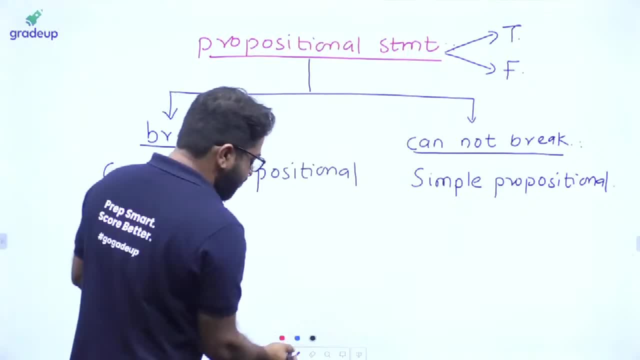 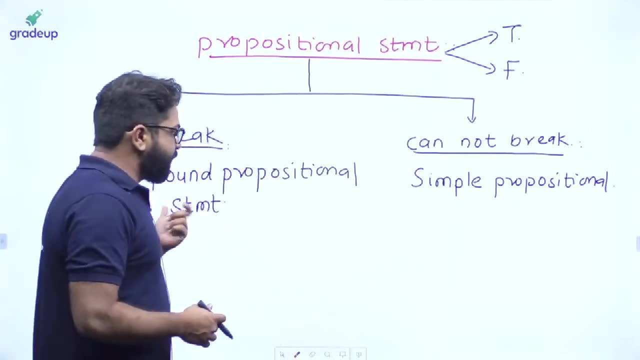 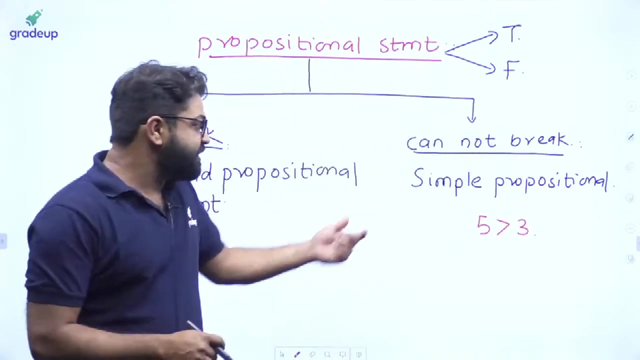 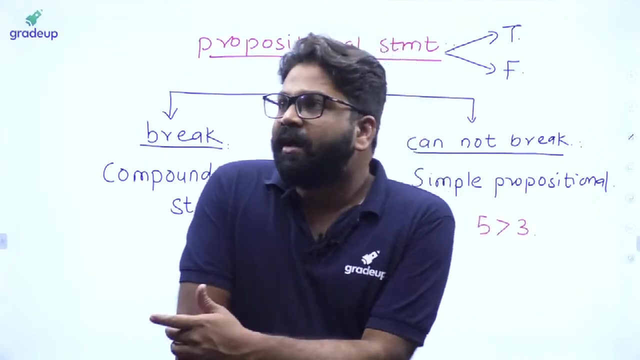 Compound propositional statement. So here you will be having compound propositional statement. Now, if I will be talking about a simple, sir, can you give me example where it is a simple propositional statement or a compound propositional statement? Let me give you that example. Suppose if I will write, five is greater than three, This is called as a simple propositional statement. Why You cannot break it. Or you may have also learned this type of thing such that you know the people are saying that Chennai is a capital of a Tamil Nadu, For example. this is a one simple statement. 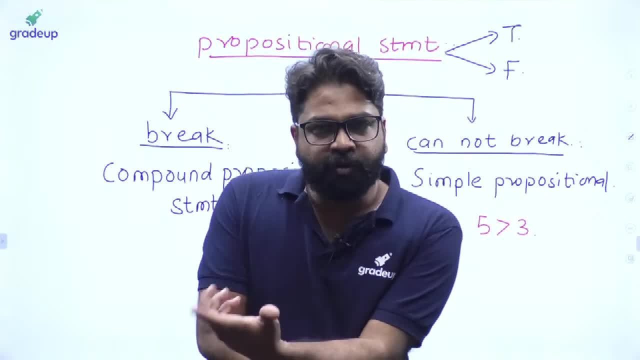 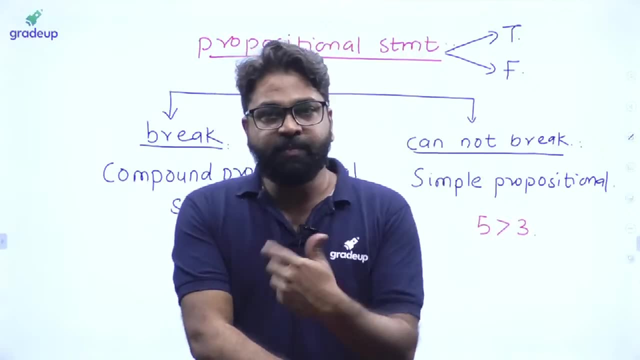 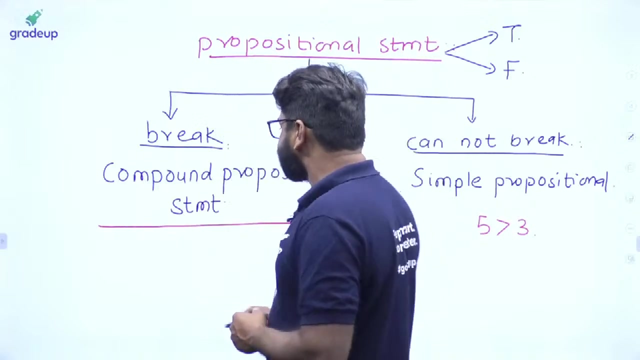 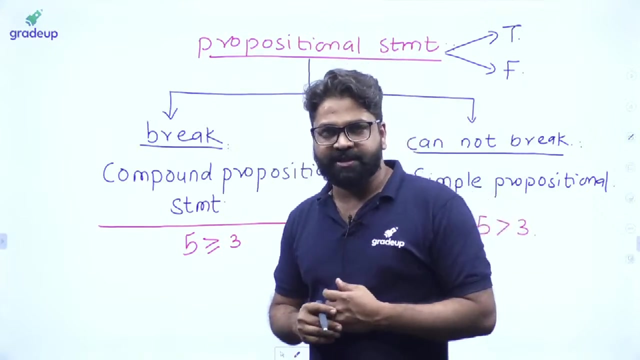 This is a statement where you cannot break it. If you cannot break it, then what will happen? That will become the simple propositional statement. But when you can break it, when you can break it, that is called as what that is called as, a compound propositional statement. So here you will be having what? here you will be having a compound propositional statement, So you will be writing: five is greater than or equal to three. See, this is called as what this is called as, a compound propositional statement. A compound propositional statement, It is a type of statement where you can break it. 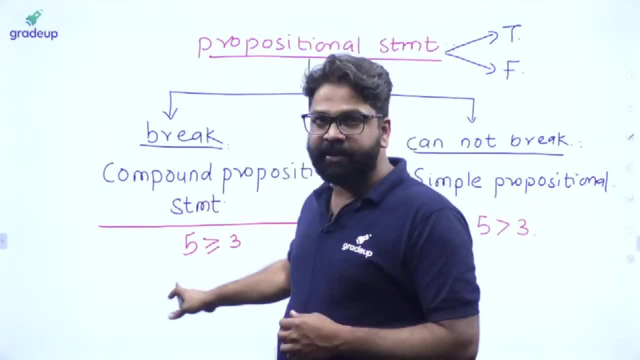 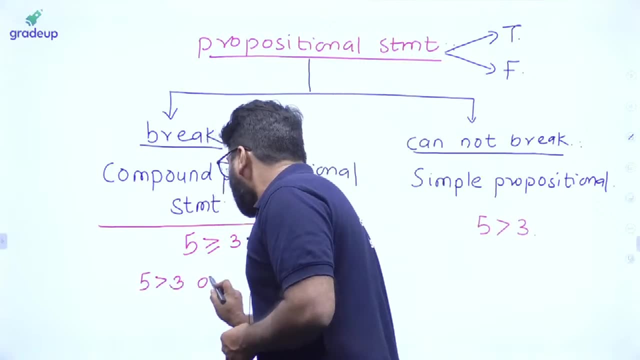 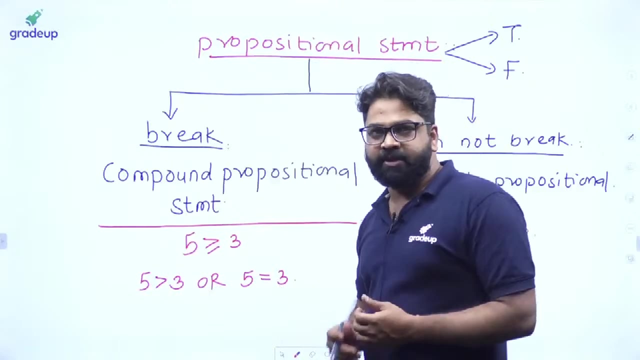 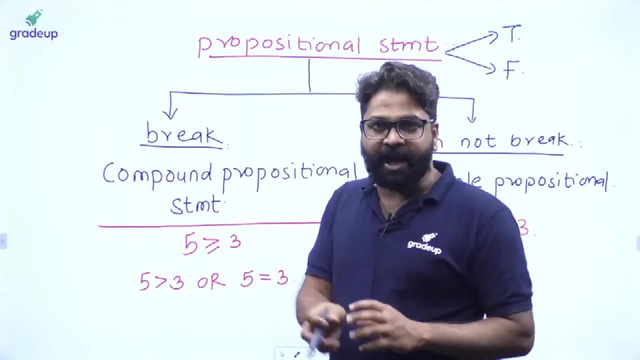 So suppose if I will write five- one example- if I will write five is greater than or equal to three, then what I can write is basically: five is greater than three, Or here what I will be writing, five is equals to three. So this is called as what this is called as a compound propositional statement, Yes or no? Now what I can write is basically here, compound propositional statement. You can break down into two or three or four, simple type of statement. So here you will be getting. 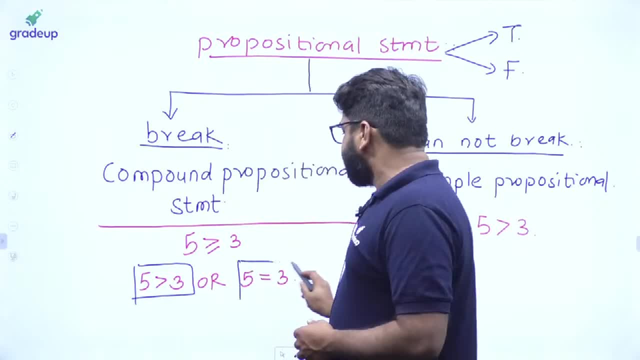 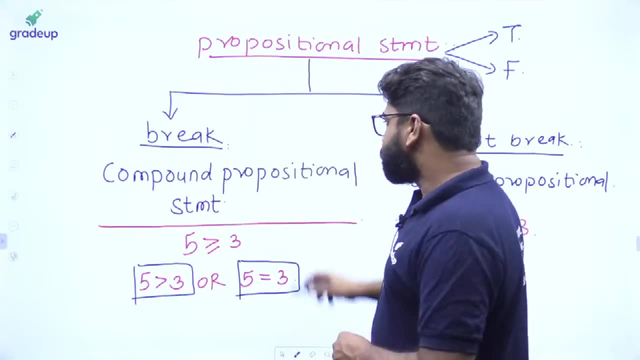 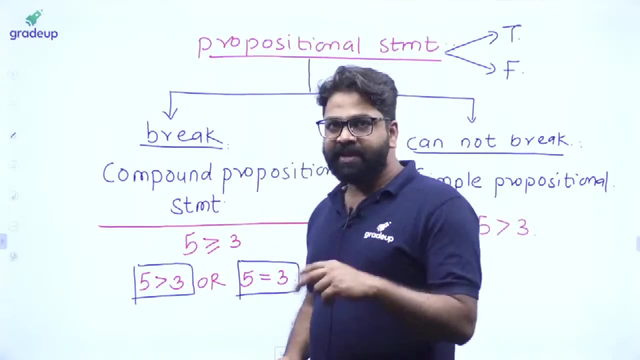 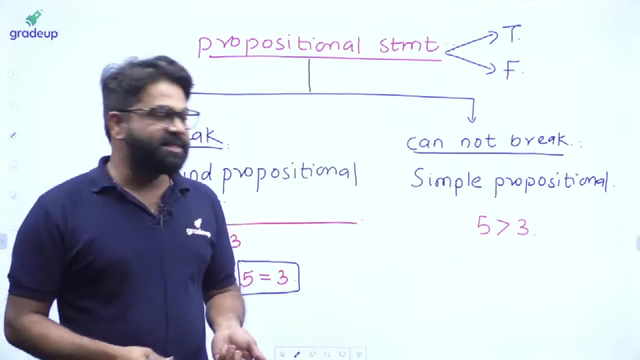 what? here you will be getting one simple statement and here you will be getting what? another simple statement. So this is the whole concepts. that is related to what? that is related to a propositional statement. So propositional statement it is of two type: One you can break it, Other one you cannot break it. when you can break it, That is called as a compound propositional statement. And then other, when you cannot break it, that is called as a simple propositional statement. So in this way we can go and we can try to understand the whole concept. Now let's go and let's. 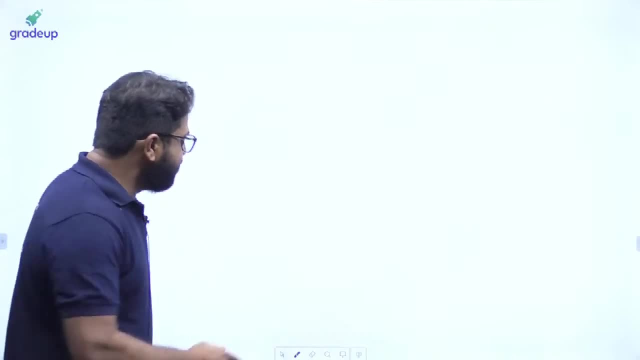 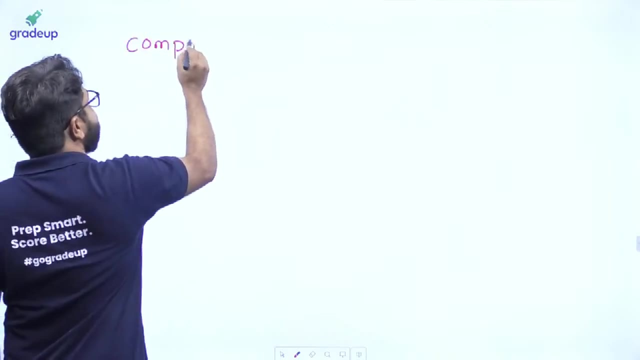 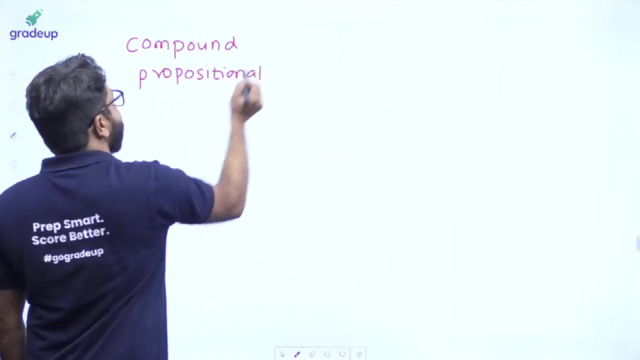 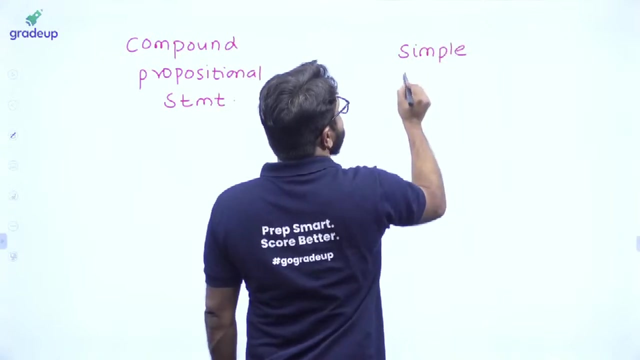 try to derive the other things that is related to that. Now, see, suppose what I will be telling you such that if you will have a compound propositional statement, Now if I will write here, compound propositional statement, if I will write compound propositional statement, propositional statement. and here if I will write simple propositional statement, simple propositional statement, propositional statement. 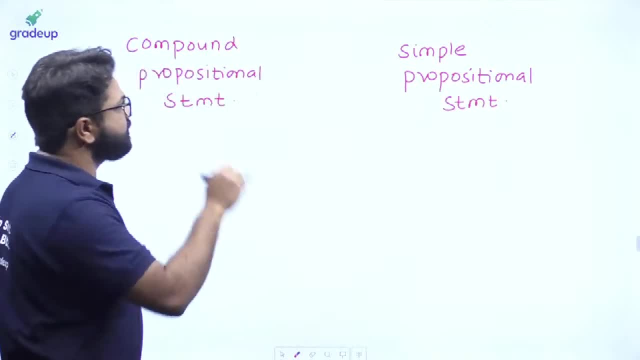 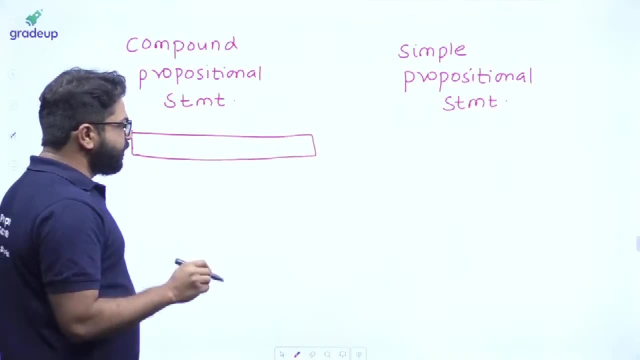 okay, so one is called as a compound propositional statement, simple propositional statement. Now, here you will be having a compound propositional statement. As we know, that compound propositional statement is, we can break down into two or more simple statement. So here you can say that you can break down this whole thing into two or more simple statement. Okay, so here you will be getting what this is: your compound propositional statement. you can break down into two simple statement. See when we are breaking 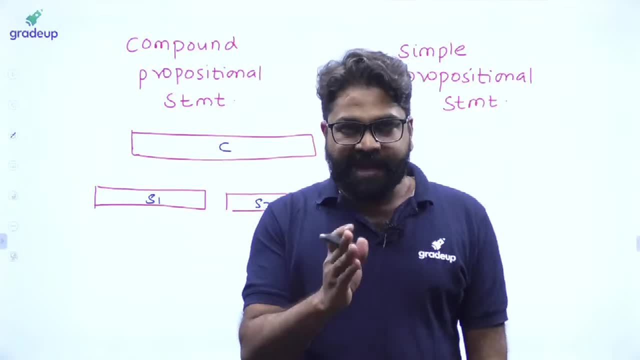 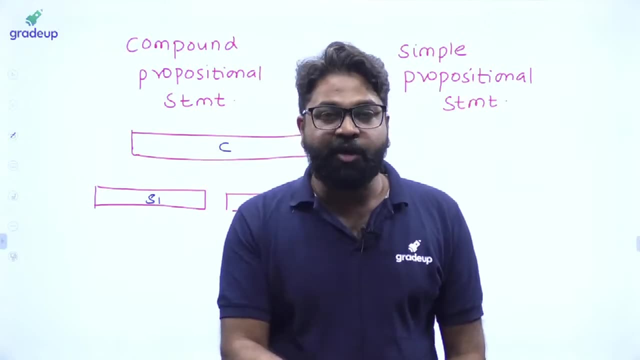 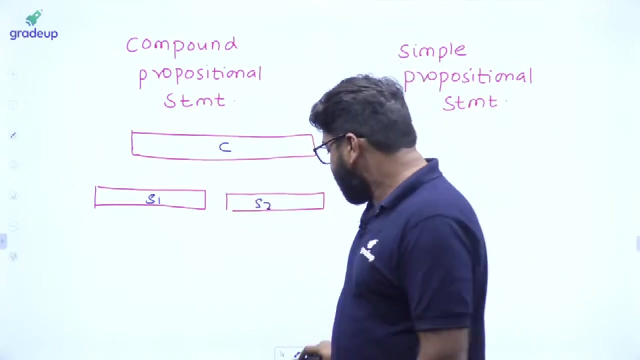 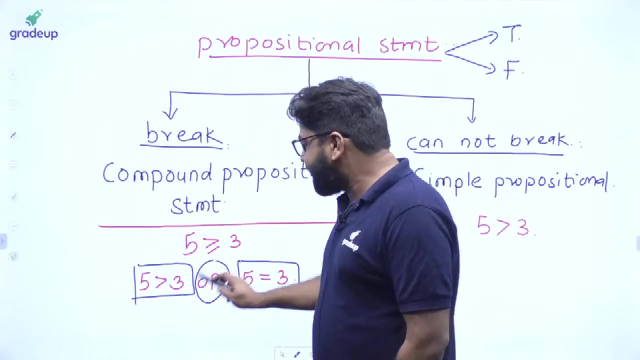 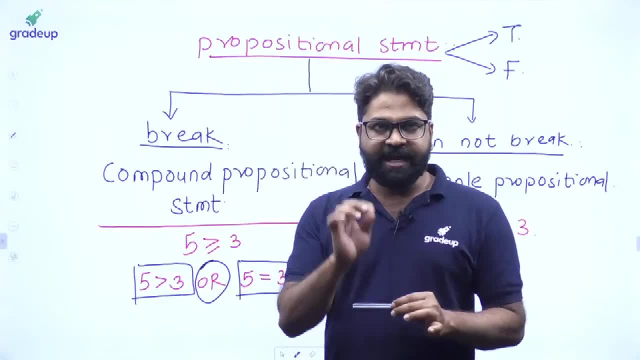 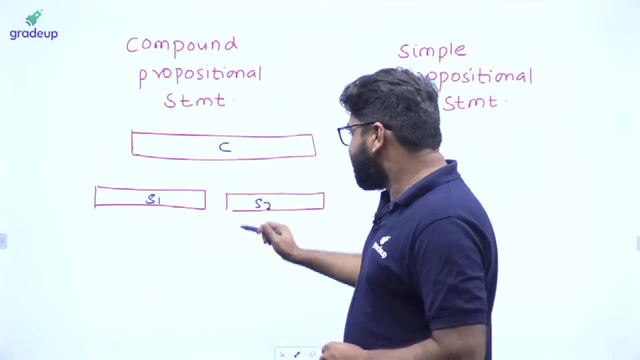 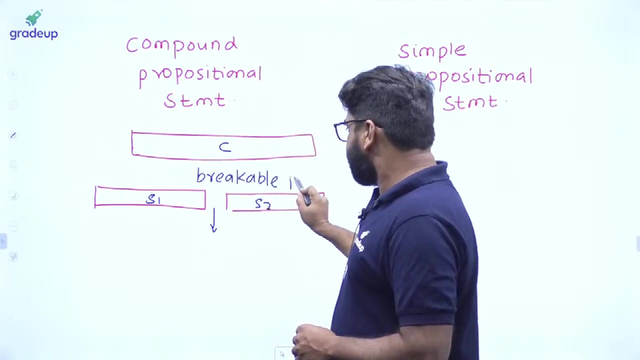 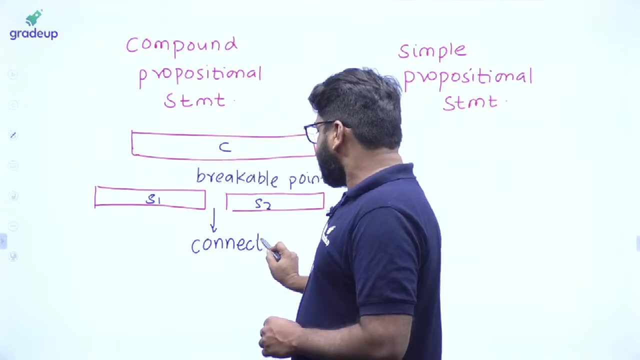 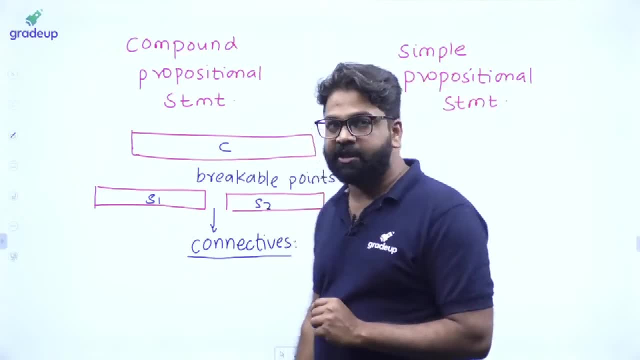 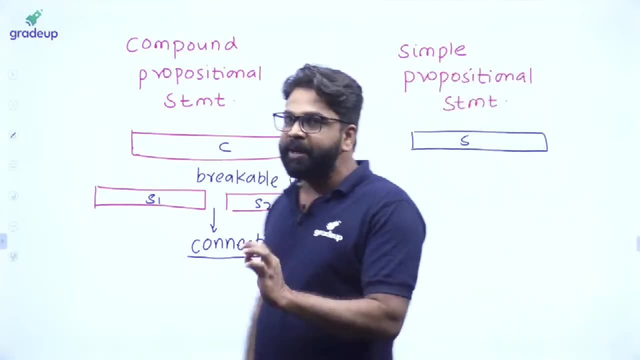 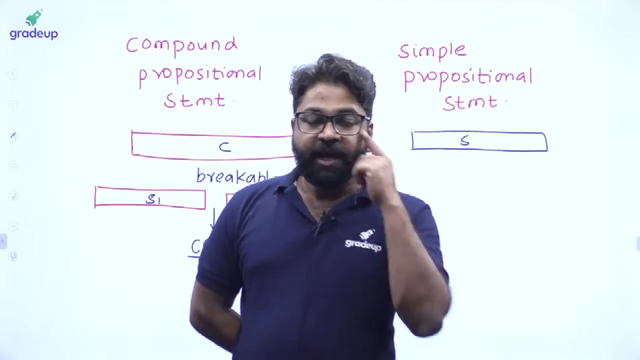 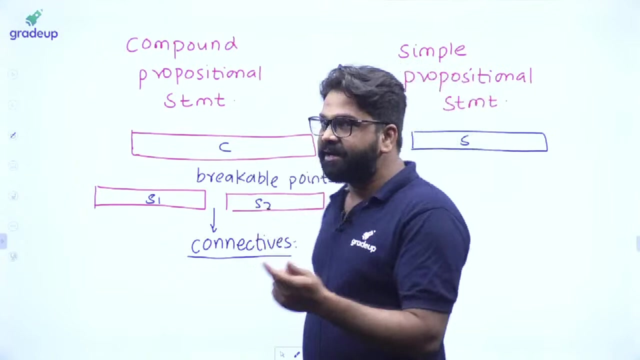 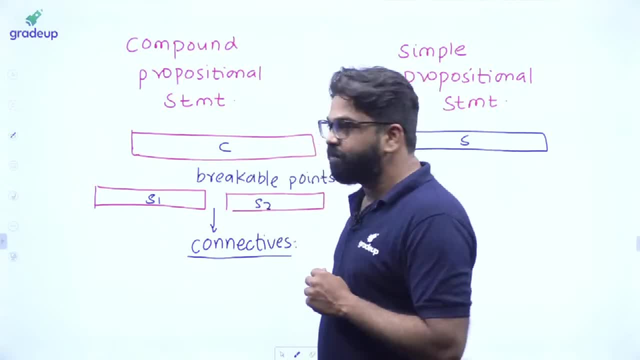 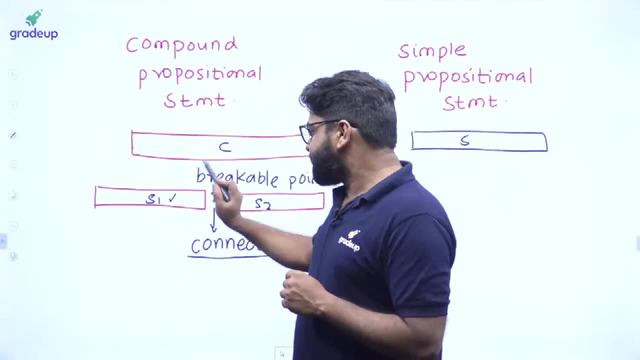 statement right now. what will happen here? this is called as a breakable points, and these breakable points are called as what this breakable points are called as a connectives right. so here you will be getting one simple statement here. here you will be getting another simple statement like: 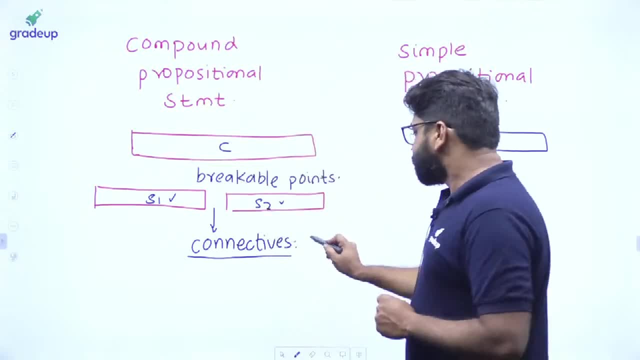 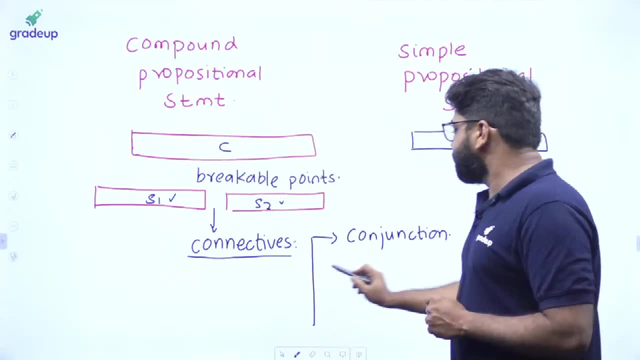 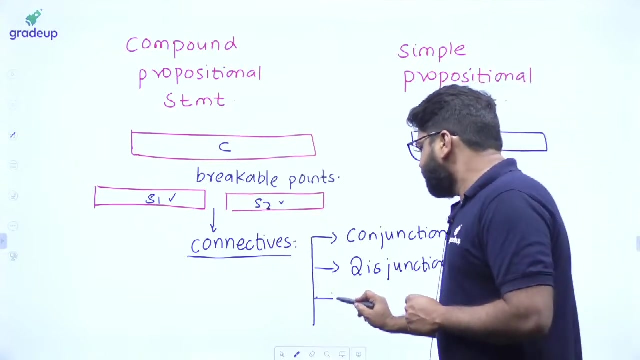 this. so we are having the four different types of connectives. so we'll go and we'll talk about that first one that is called as a conjunction, so here this is called as one connective. another one that is called as a disjunction, so this is another. you can say that connectives, and then we are having a. 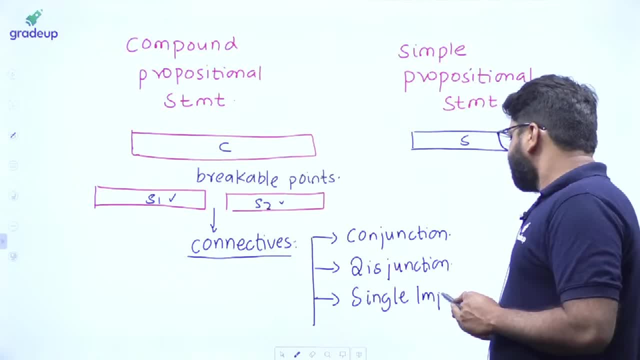 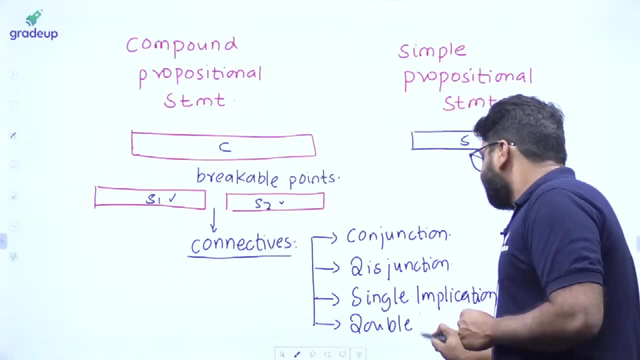 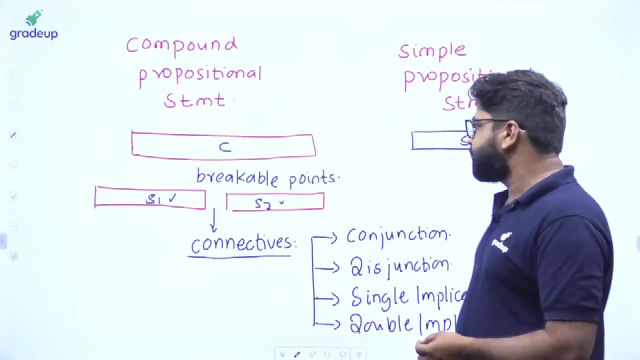 single implication, single implication, and then we are having what, and then we are having a double implication. this all are the different connectives that you people are having, so one is called as a conjunction, disjunction, single implication, double implication. sir, i also heard that, which is nothing. 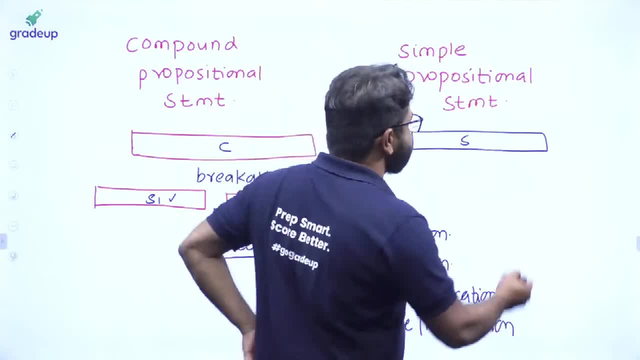 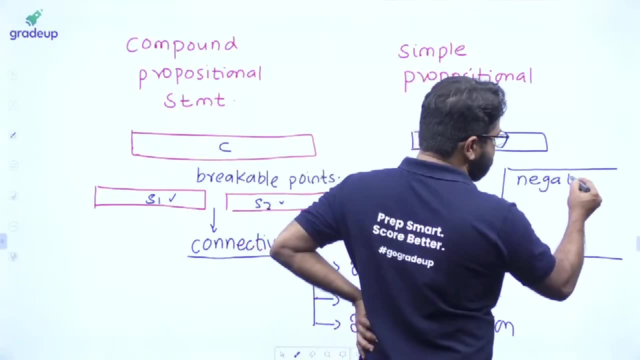 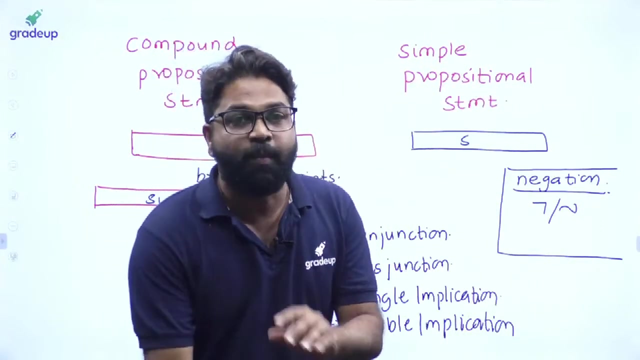 but you can say that modify, or you can say that negation- yes, negation is also there, but negation is not the connectives. negation is basically what negation is called as a modifier. so here i will be writing this negation sign like that. so negation is called as what negation is called as a modifier. so which negation? 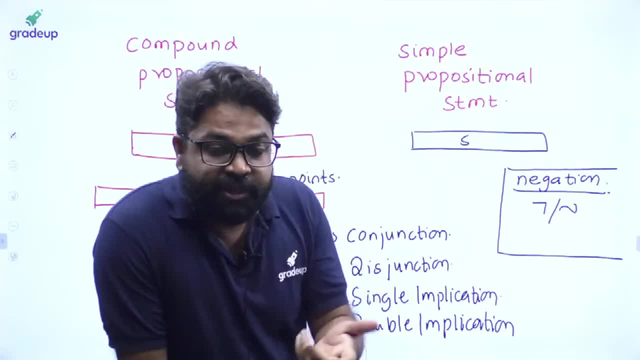 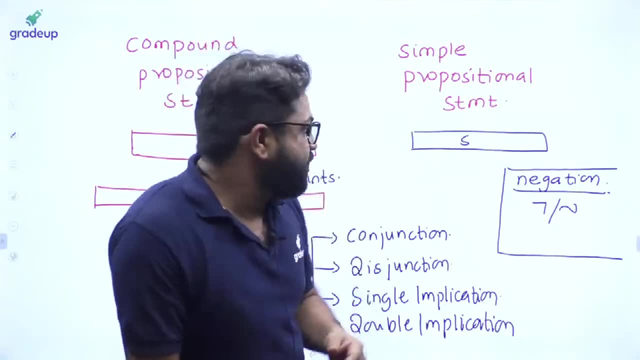 does not okay. negation does not connects two or three simple statement. what the negations does, negation modifies the statement. so negation is also called as what. negation is also called as a modifier. so here you will be having what, here you will be having the. 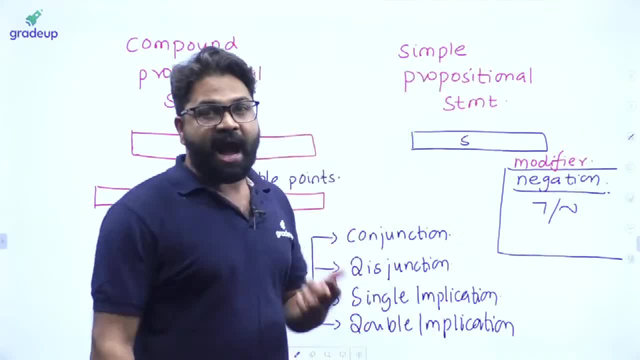 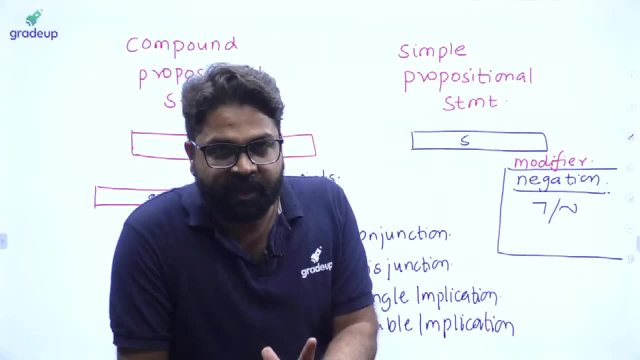 modifier, so it modifies a simple statement. einstein is a genius. einstein is not a genius, so it modifies a statement. it does not connect two or more simple statement, right? so that is nothing. but this is the whole concept that you'll be having. one more thing, see the very importance. 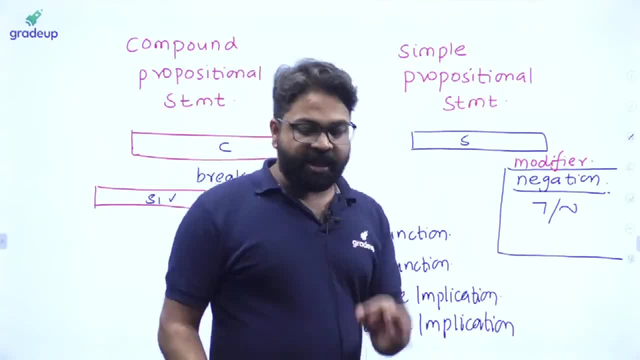 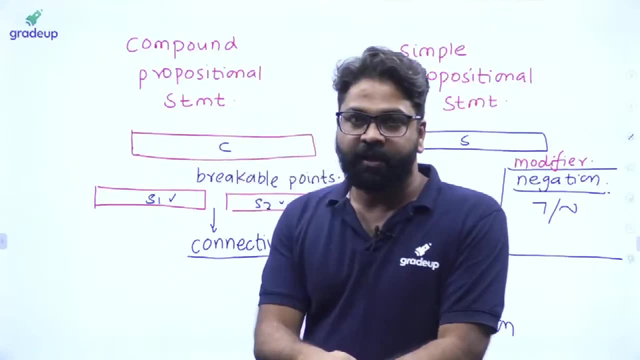 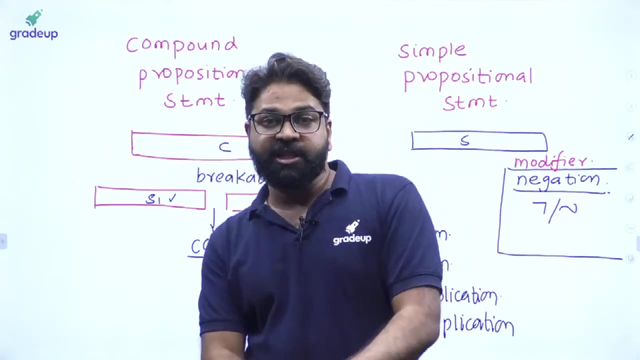 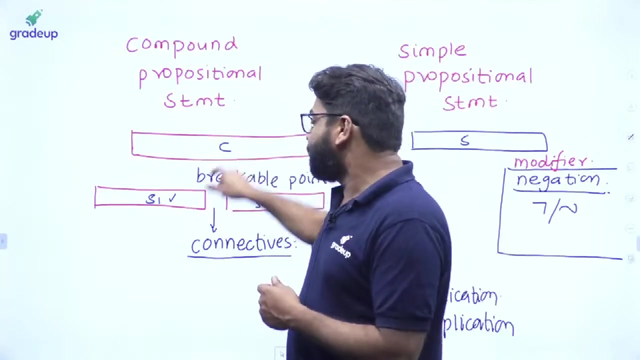 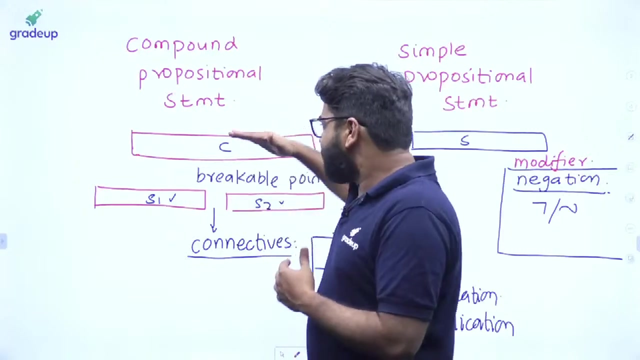 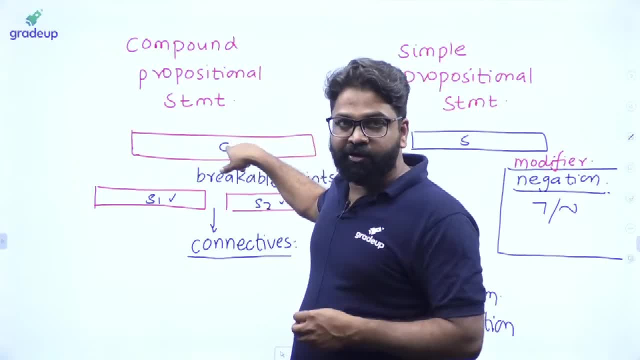 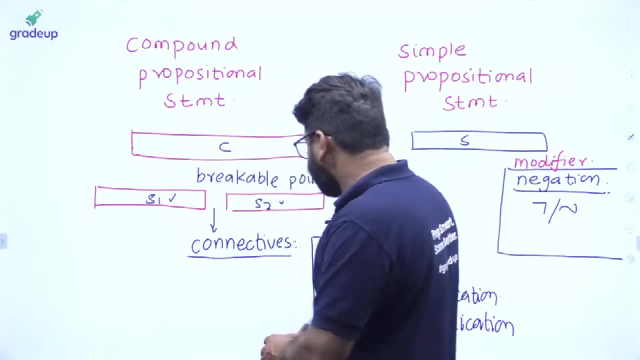 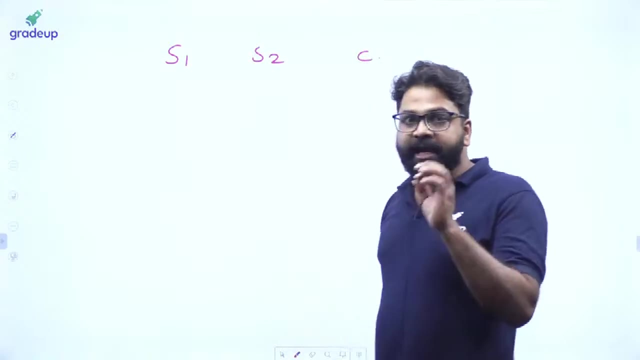 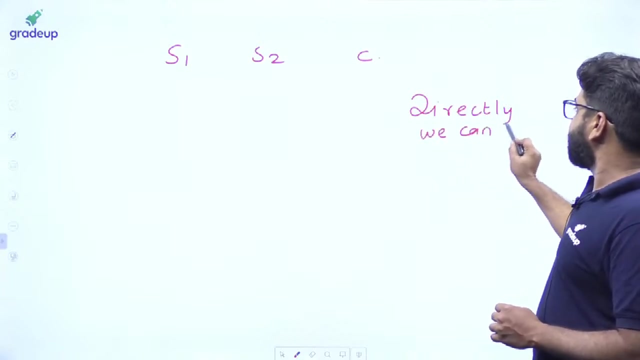 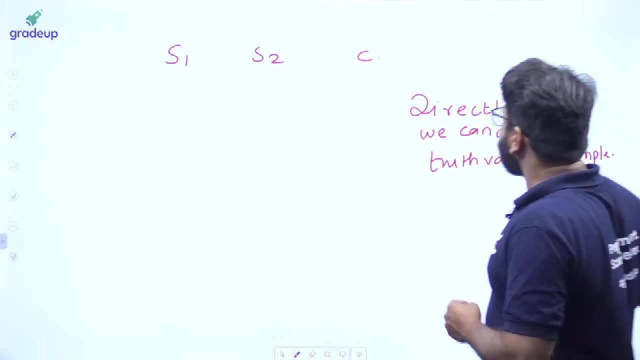 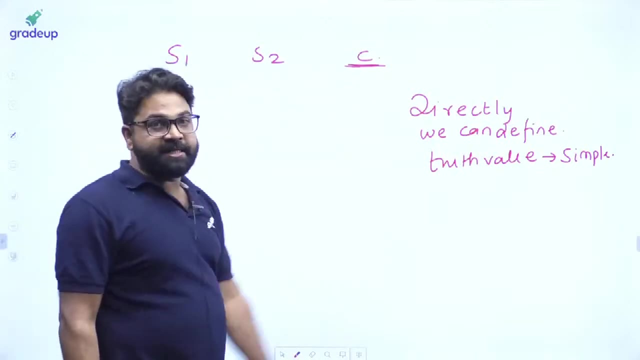 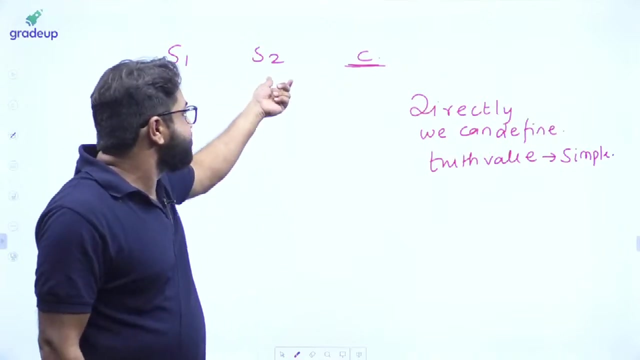 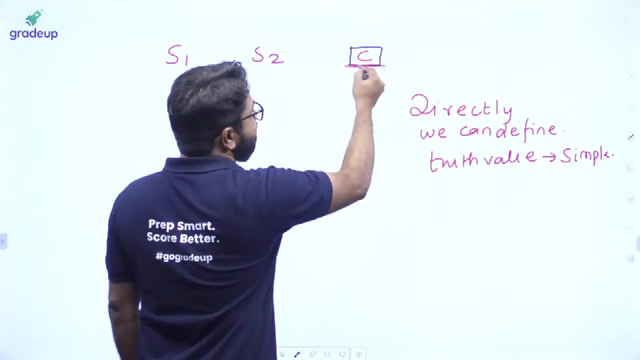 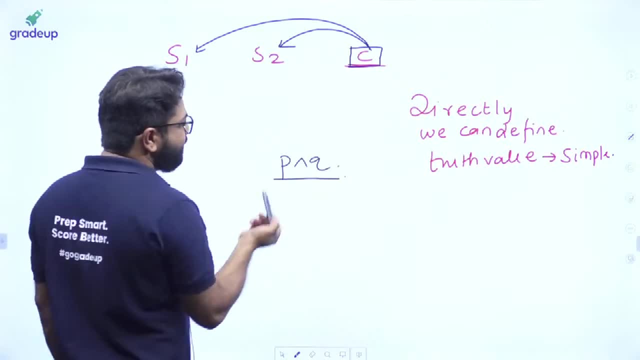 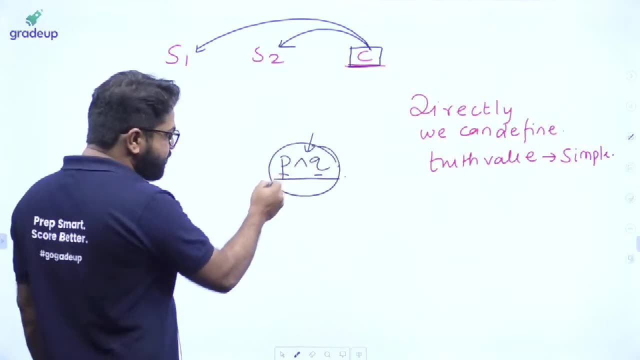 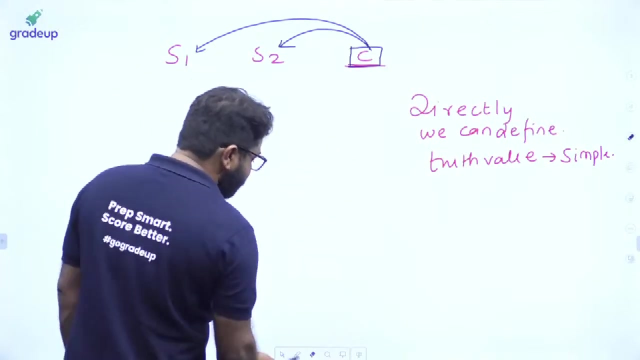 right. see, this is a compound propositional statement. you know why this is one simple statement. this is another simple statement. this is connective. so when you want to define the truth value of this, it is dependent on P, it is dependent on Q. that is nothing but my point, or the observation. now let's see. 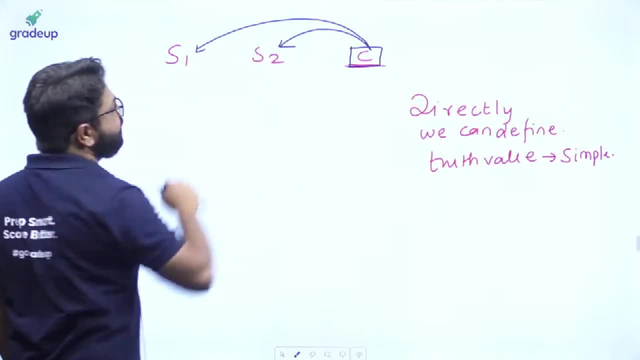 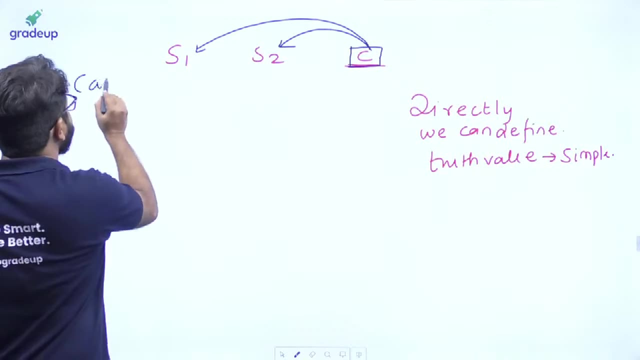 this. so what will happen, sir? obviously, when it is dependent on that, then you will be getting a cases, yes or no, then you will be getting a cases. yes, then you will be getting a cases. so here I will be getting, which is nothing but case number one. what will happen if both will become a true? so here I'll be having a. 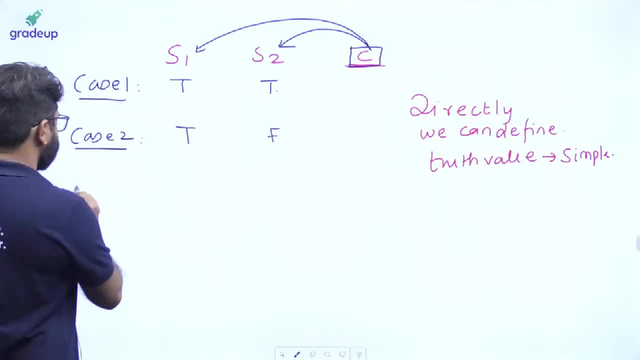 case number two. what will happen if the first one is true, second one is false. now here I will be having a case number three here if it is a false, and then it is a true, now here I will be having a case number four. so if it is false and 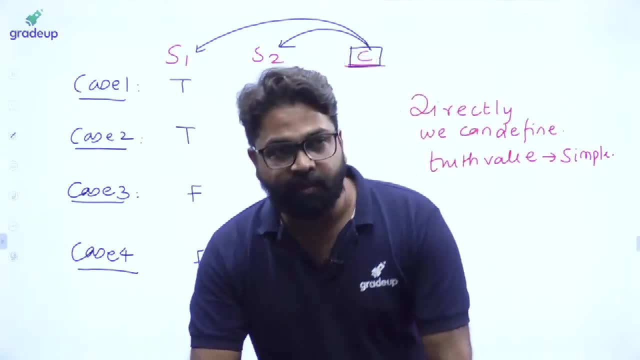 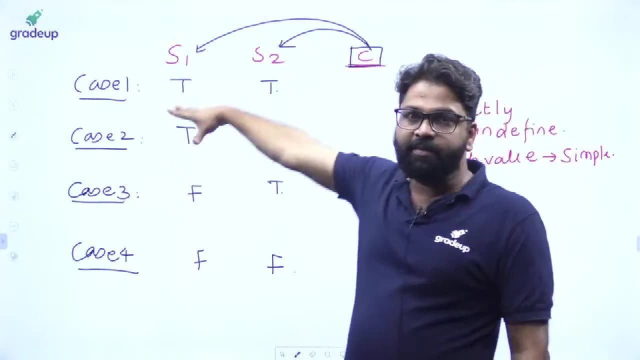 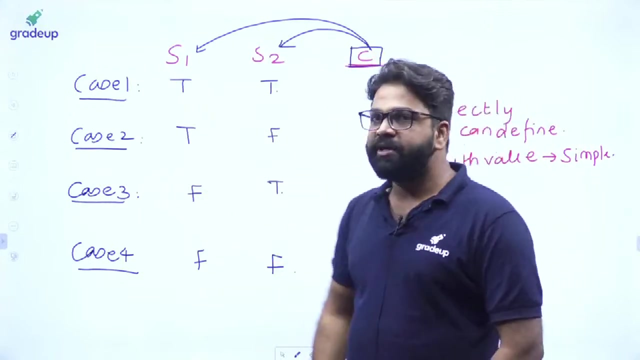 if it is a false. so basically, truth table is nothing but a case studies of simple propositional statement. so the compound propositional statement is totally based on simple propositional statement. so if anybody is asking what is a truth value, then you have to say that a truth value is basically defined as what a truth value is basically. 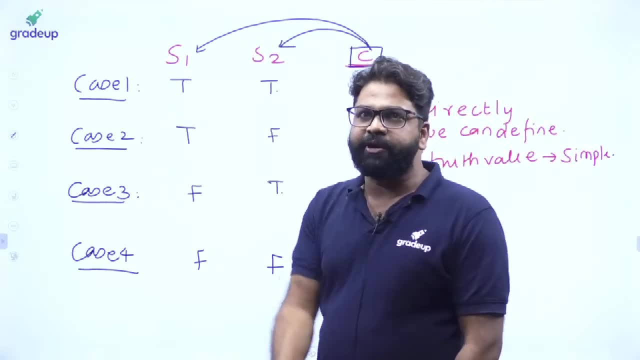 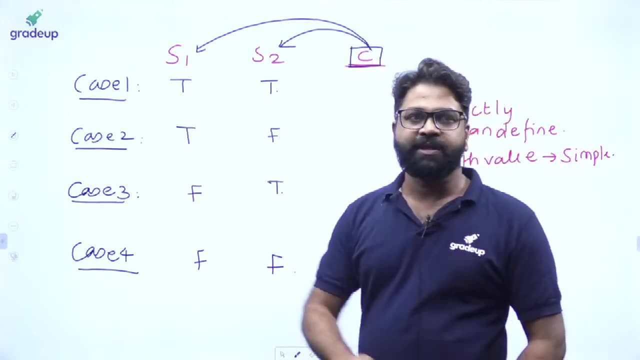 defined or truth table. if somebody is saying that what is the truth table, then you have to say that truth table is basically a case studies in order to define the compound propositional statement. so that is nothing but the whole concepts that is related to that. okay, so that's it for the today and we'll 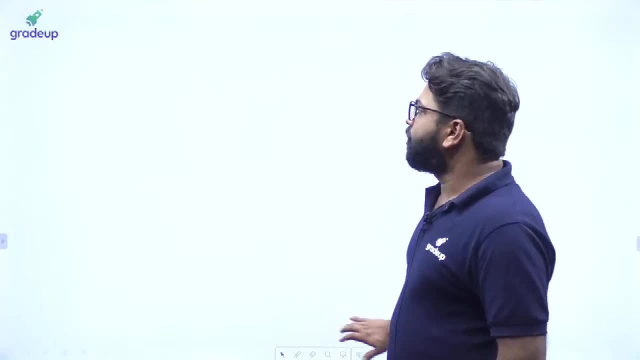 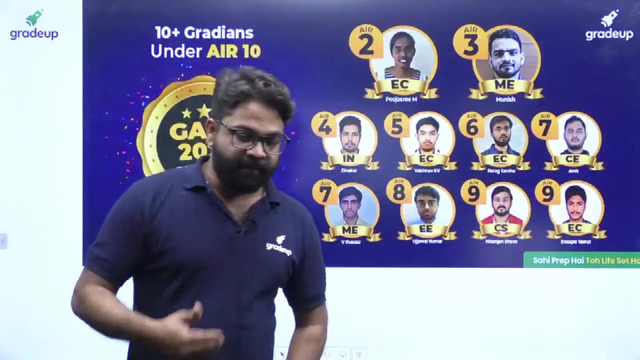 go and we'll talk about the other sessions. okay, we'll go and we'll talk about in the next session we will be talking about the other things, but before that I'll tell you these all are the rankers. so if you want to prepare with the grade up, you can take a- you know- grade of subscription and this all. 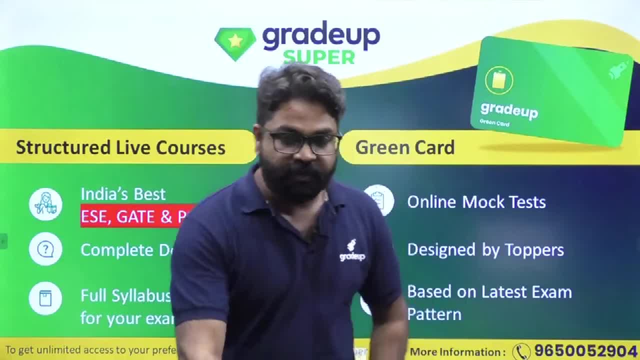 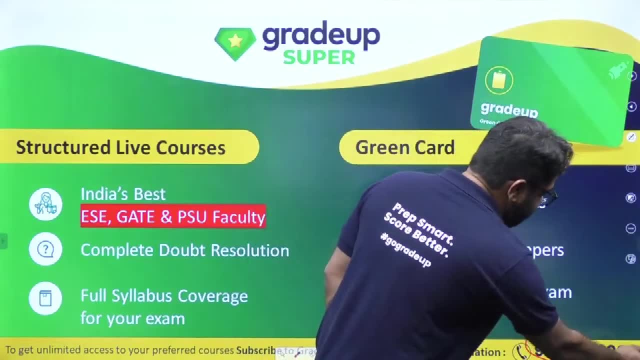 are the advantage that you people are having with respect to what? with respect to the gate of super subscription? now, if any person wants to have the assistance, then that person can contact on this particular number, such that nine six five zero zero five two. nine zero four. so in. 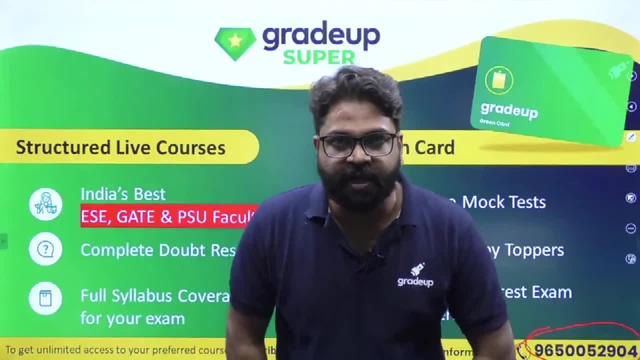 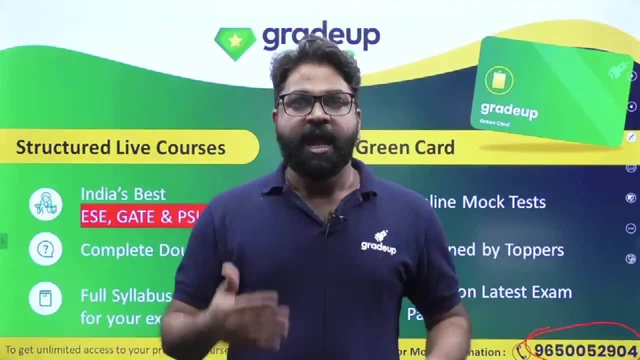 this way you can have all the subscriptions that is related to that. okay, thank you so much, guys, for coming on this particular session and then we will be having the- you know, the certain sessions, and every day at 5 o'clock I will be having- you know, you can say that- practice session on a grade up app and 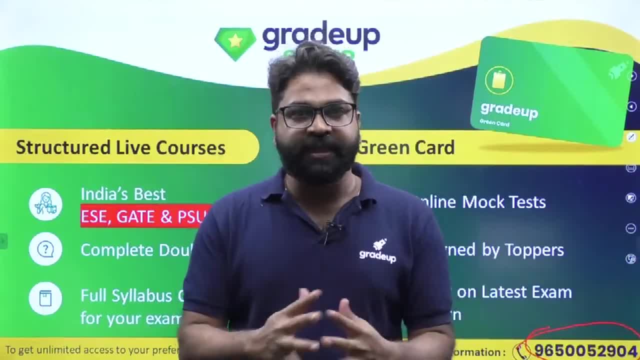 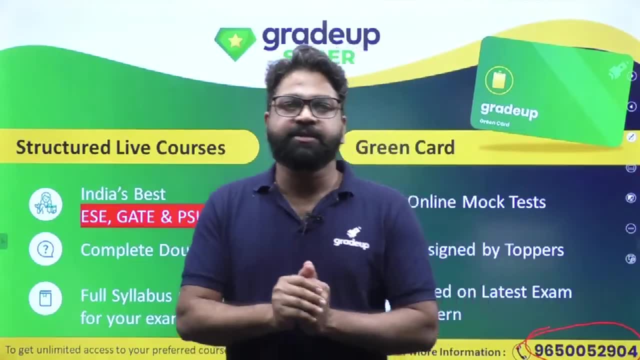 it's totally free. so if you wish to join, you download the grade up app and then you follow me over there and then you can come and you can join the practice session. right now the graph theory practice sessions are going on, so you can join at that point of time. okay, yes, thank you so much, guys, for listening.